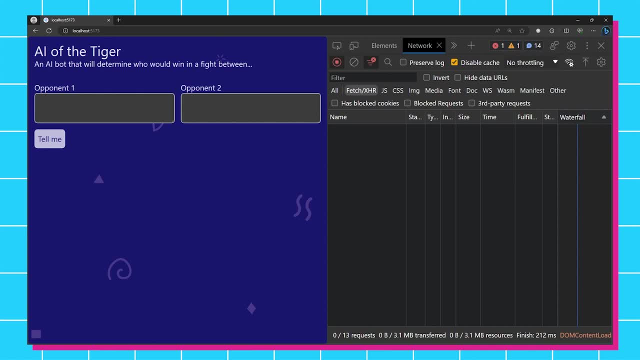 necessarily having to have an idea and just have some silly options to choose from. I also want to add a little disclaimer that you know this app is built with AI, so it has a couple of little quirks and wonky things about it, And then I think it'd be a cool idea to include 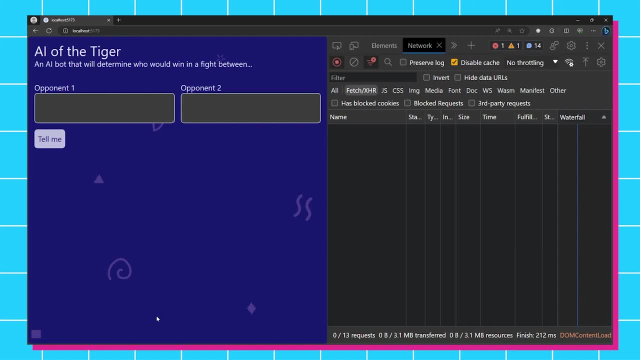 a shout out that you know I made it and it's hosted by Akamai And we'll have a little link to a promo for $100 of Akamai Cloud Computing credits. So I'm going to do that first and then. 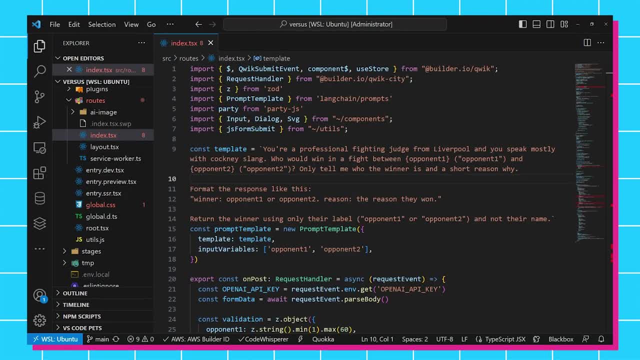 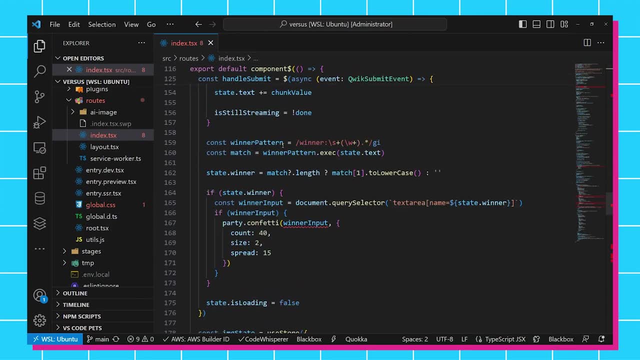 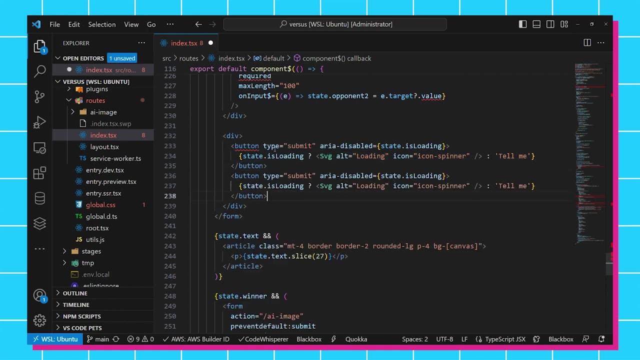 we'll work on the deployment. So, going into our application, let's start by adding the button that was talking about. Okay, so in the component, I'm going to scroll all the way down to the template where we have the submit button here, And I'm just going to duplicate that for now, because I know. 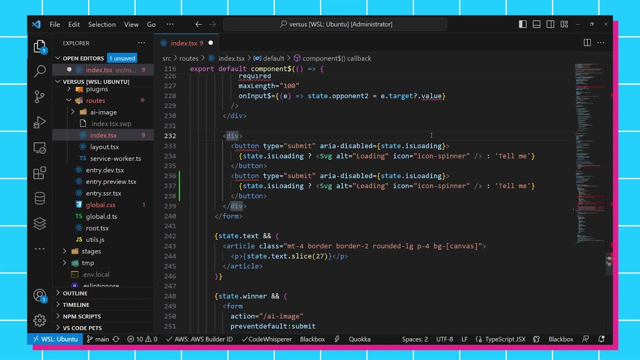 we're going to need two buttons, And because they're next to each other, I want them to be sort of side by side. So we're going to say: this is not going to be just a div anymore or display a block, This is going to be a display of flex And I want to have a gap of four. Okay, now here. 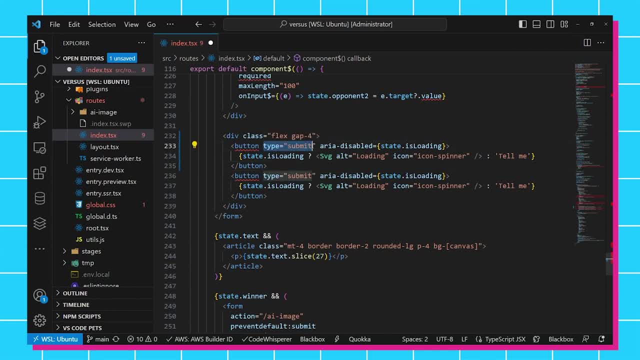 though with this first button we can leave the type of submit. This is optional because the default button type is submit. Here we want to be explicit and set the type to button, because we don't want clicking this one to submit the form. Next we'll get rid of that And then we can get. 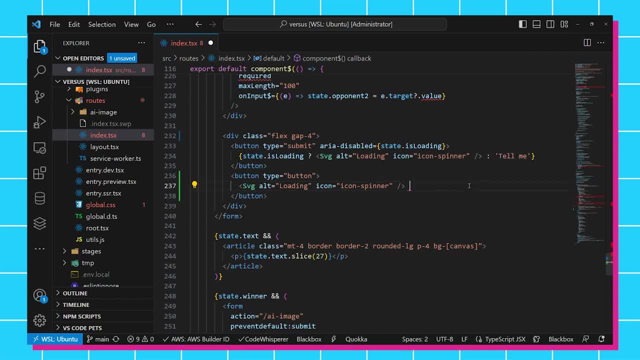 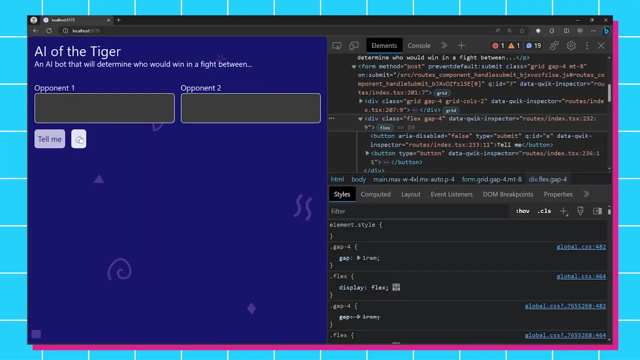 rid of this. I am going to leave the SVG there, because my thought is we'll have something like this. It looks pretty good, So then you can click this. I'm going to replace this icon And I want to have it with the SVG, And then I'm going to click this, And then I'm going to click this And. 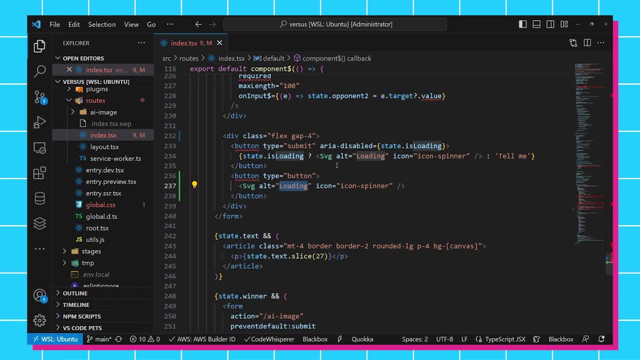 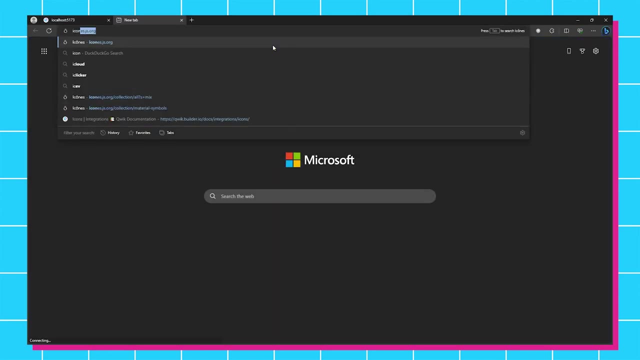 it's something that's like a random selector. So instead of the alt text being loading, this is going to say pre-fill: random fighters, something like that. Okay, so now we need to replace this icon And we have a really handy setup for working with icons. So I'm going to go to icons And I'm 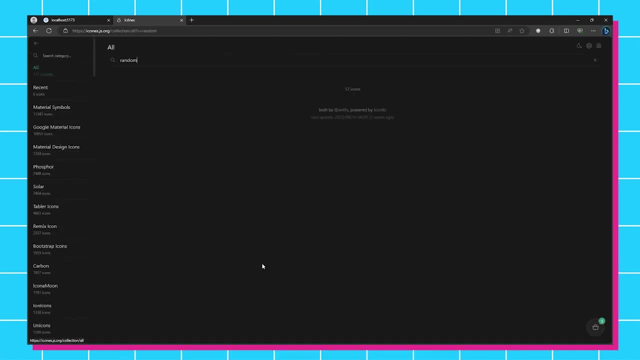 going to search for random control. enter to search the entire library And then we have all these to choose from And I kind of like this. I'm going to click this little card. Well, maybe that, maybe this mystery box? No, I'm going to. 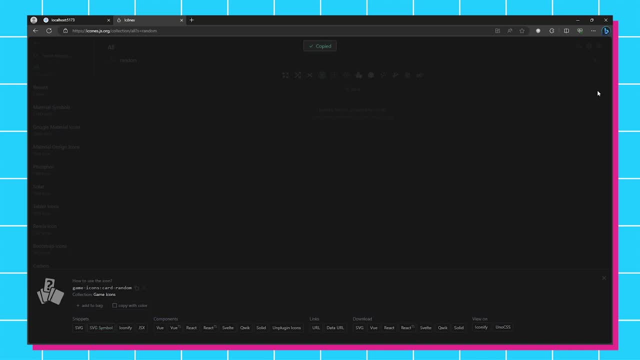 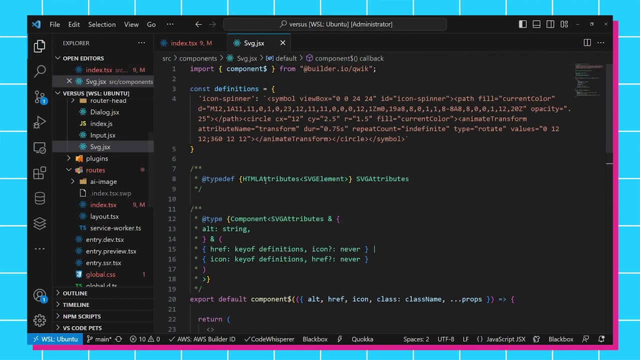 pick the cards. Sure, We're going to copy the SVG symbol, going to close that and go into my SVG component And we're going to update our definitions here. So we're going to add one called icon- random, I think- And then we will paste in the symbol Whoa that we copied, And then I just 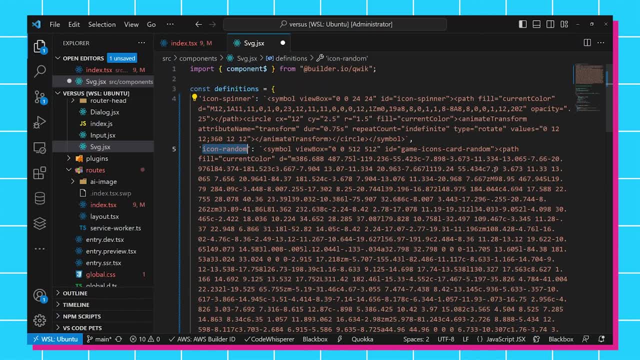 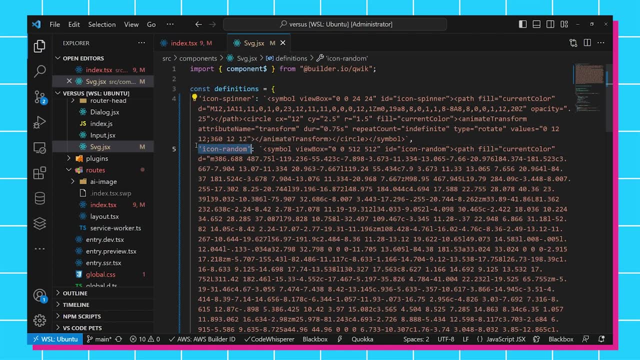 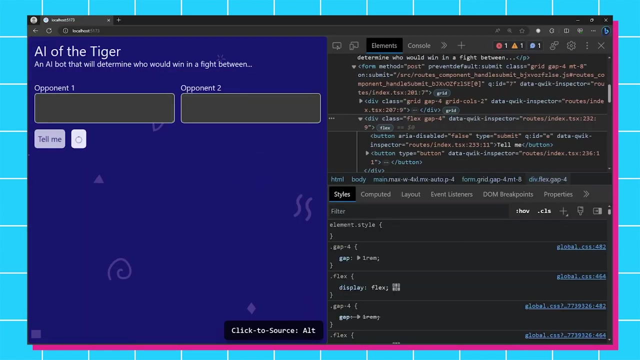 need to make sure that this key matches this id. so the key is what's going to be used to tell typescript what options are available, but the id is going to be the actual thing that tells the html markup what the svg should be. so close that, uh, yeah, that's right. actually, we forgot to do one thing we have to. 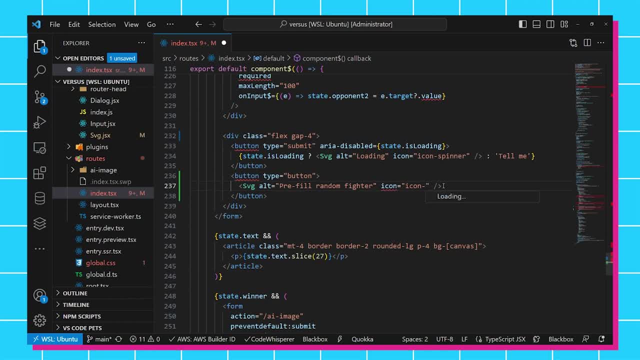 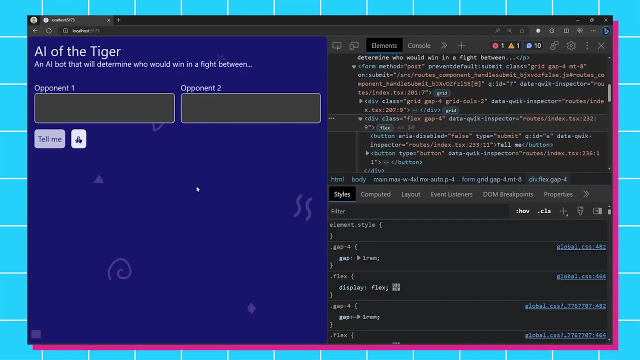 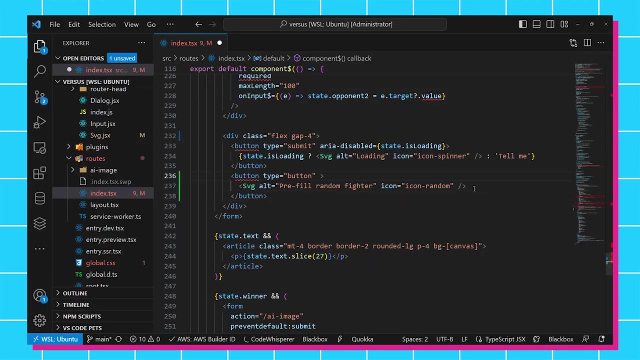 actually change it here. so now instead of icon spinner, we have icon dash and we have random as the option. there you go, there we go. how about that? that's pretty cool. and then i'm going to add one more little little touch here that uh for visual users. they might want to hover over that. 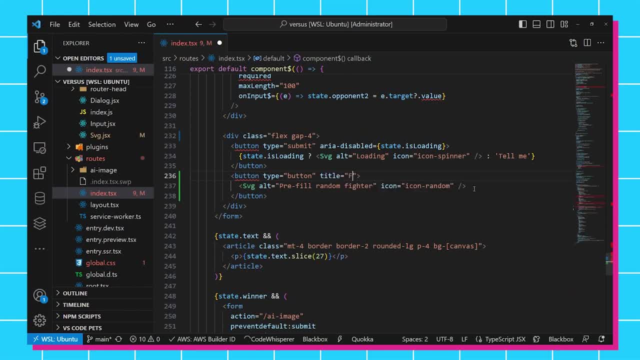 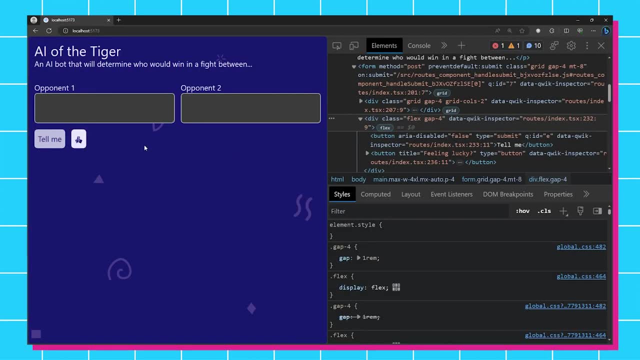 and see something. so we're going to say: a title equals uh, just feeling lucky. okay, so now hover over that feeling lucky, bam. now we have to make it actually work, you? so i want to have a click event listener for when this button is clicked for to do something. so 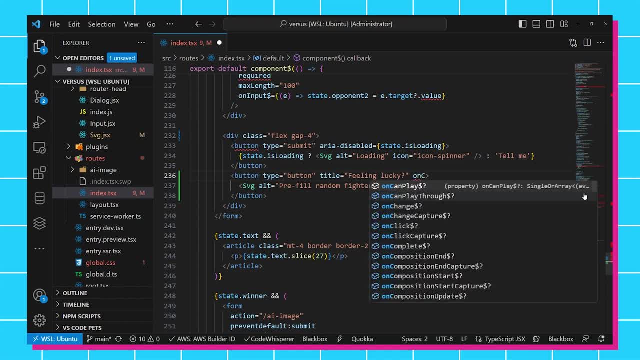 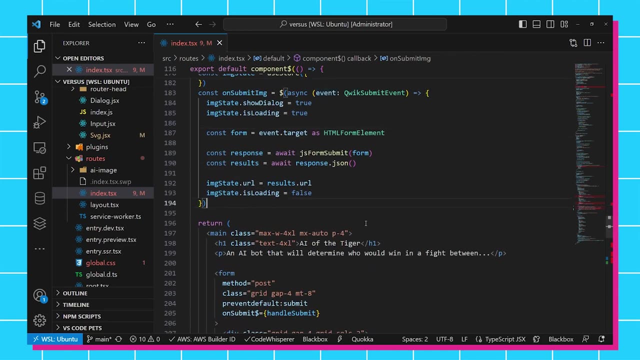 we're going to start with just adding the event listener, so on, click, and we're going to call this: uh, pick random fighter fighters, something like that. it's not defined yet, so we have to define it, so we're going to go up into our component. uh, i think i'm just going to put it here, down here at: 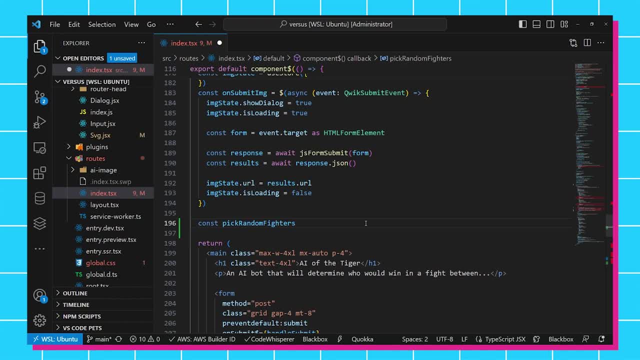 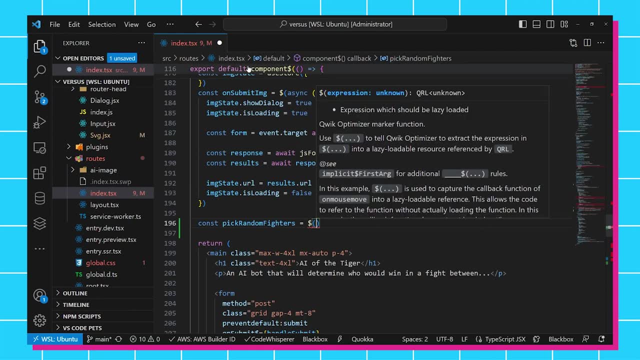 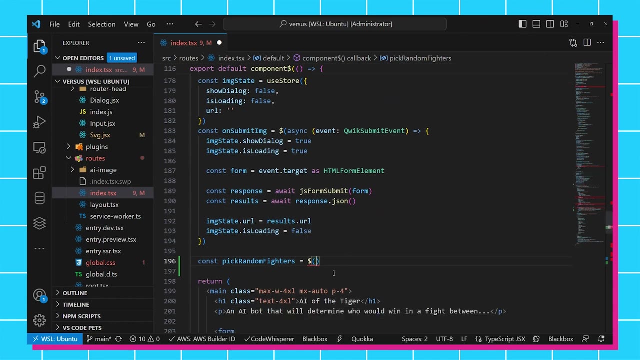 the bottom and we're going to say: const pick random fighters going to equal once again. this should be familiar. uh, we do the dollar sign parentheses and then we can put whoop, there we go, uh, and then we can put our event handler in there. so i don't think i need access to the event, i just want to execute a. 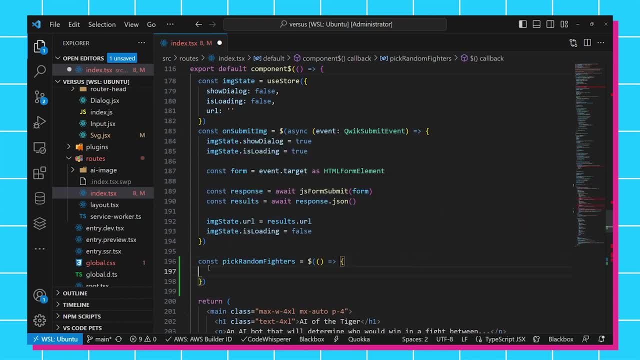 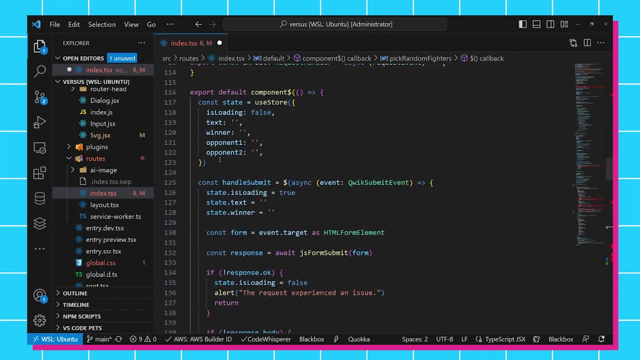 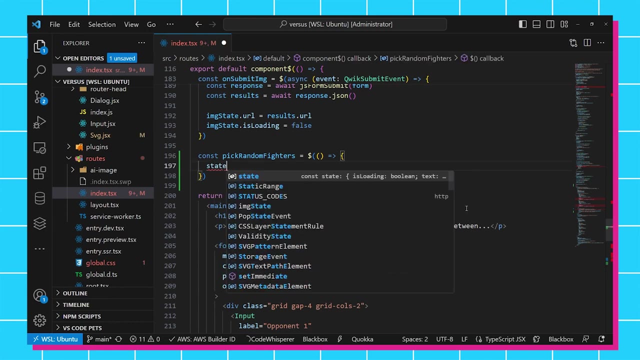 function and inside of the function, what are we going to do? we are basically going to assign random fighters to the state uh dot opponent one and state dot opponent two. so let's just start with that. let's say state dot opponent one is going to equal. for now we'll just do bigfoot and state dot opponent. 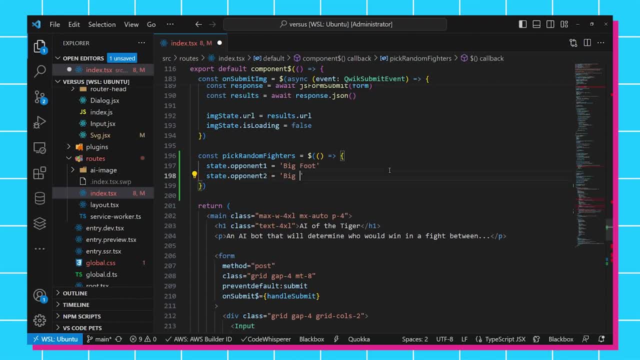 two is going to equal. uh, nessie, so let's see if this works. click that, boom. so now we just need to actually implement randomly selecting these, and for this part, i'm just going to be copying and pasting from a list that i've already created: uh, you can use your own list, or you can go out and 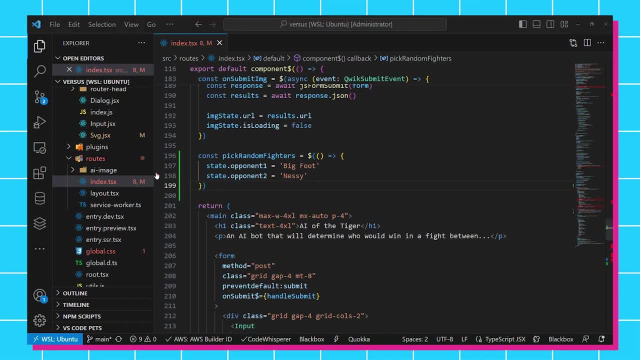 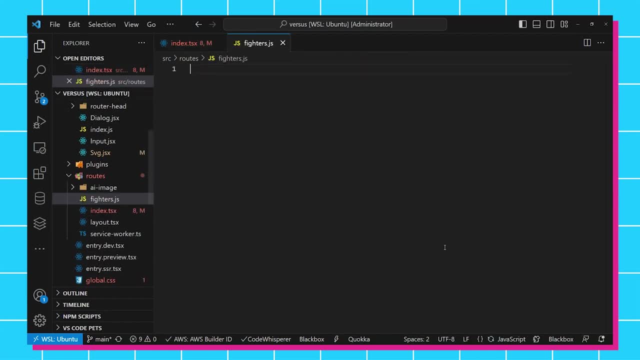 go ahead and go to the github repo and copy the file if you want. so just next to this file i'm going to create a file called fightersjs and i am going to export default this list of fighters that i've created. it's an array where we have mythological cryptids, fantasy, sci-fi, people. 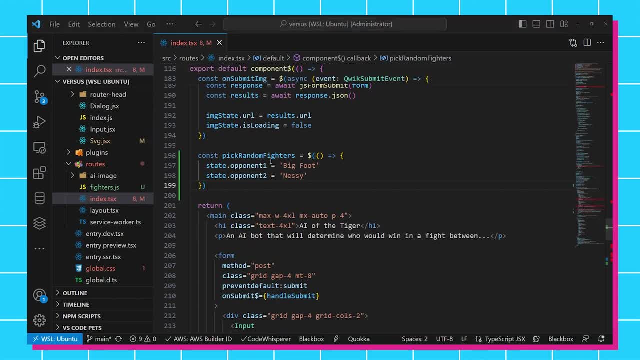 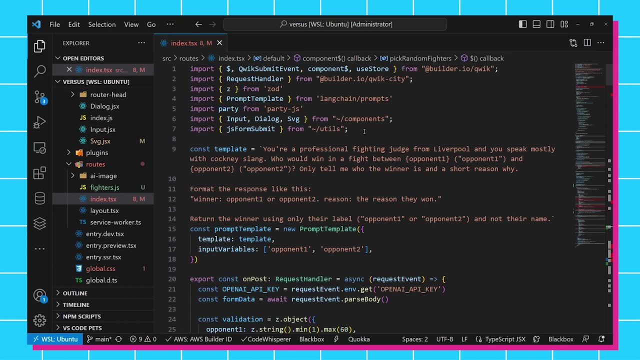 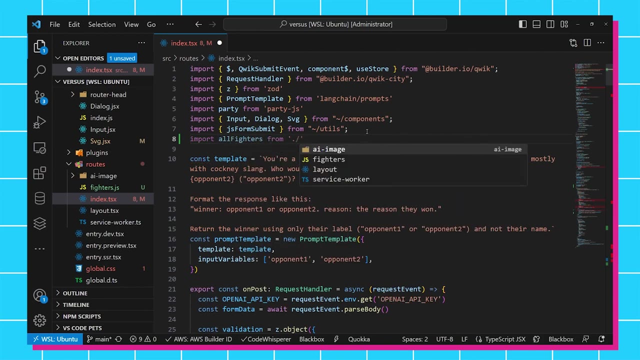 animals should be a fun list. now i'm going to import that list of fighters so we can actually work with it. so we're going to come in from, let's say, here i'm going to import all fighters from dot slash fighters, dot js. so once we have these fighters we need to 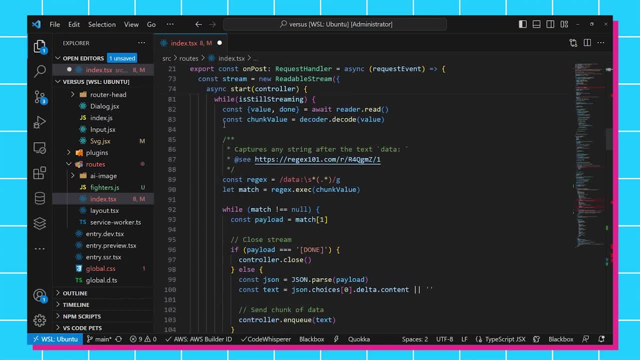 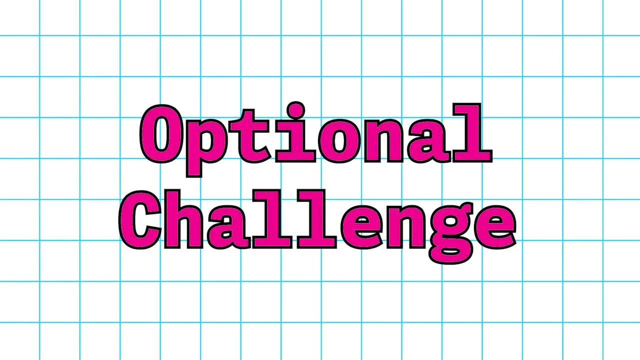 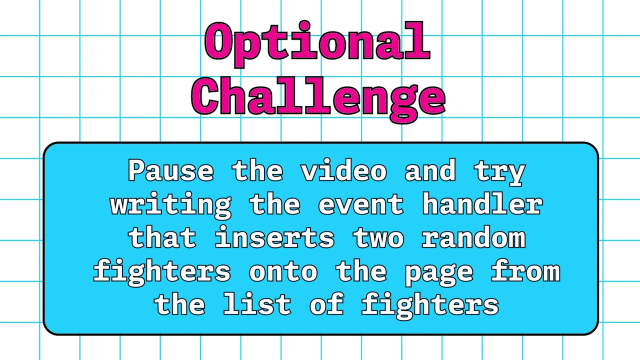 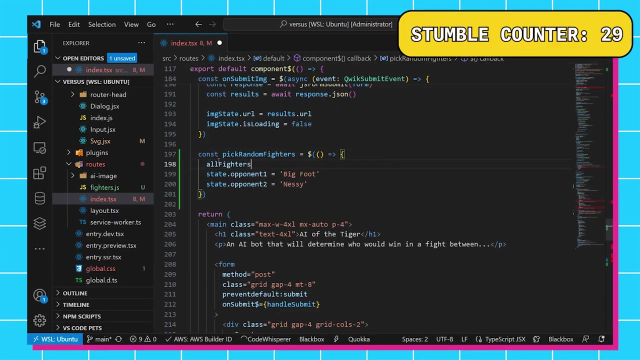 implement actually randomly selecting them. so i'm going to go down to my component where i was working. here it is and now the tricky thing is we essentially want to rent, select a random uh fighter. we want to select two random fighters from the list, but we want to make sure that there's not a chance that. 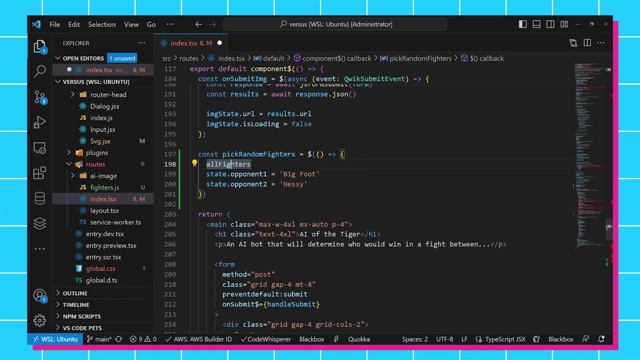 we accidentally select the same fighter. so what i'm going to do is actually duplicate this array. i'm going to say, const fighters equals, and then we'll just do a shallow clone of the array. whoops, there we go. and then i have one that i can modify. and if i modify, 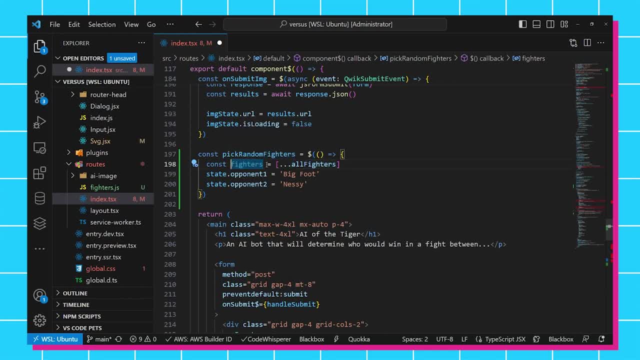 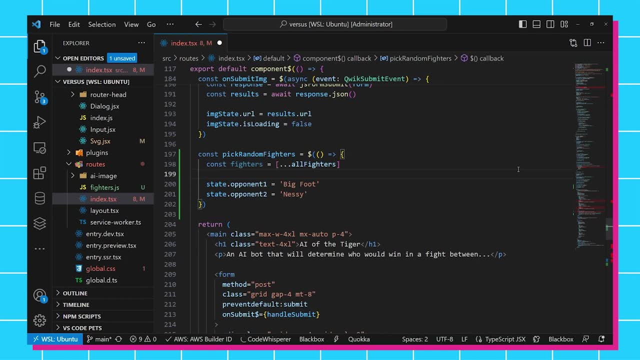 this one. i can basically pluck one fighter out and leave this as a mutated array, and then i can pluck the second fighter out and know that we won't have any sort of conflict. so the way i'm going to do that, i'm going to say const index one is going to equal math dot floor, and then we'll do. 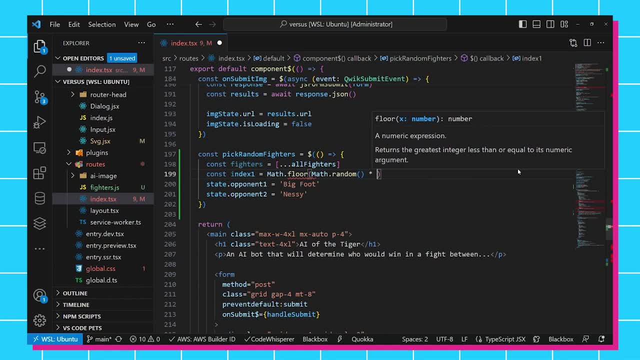 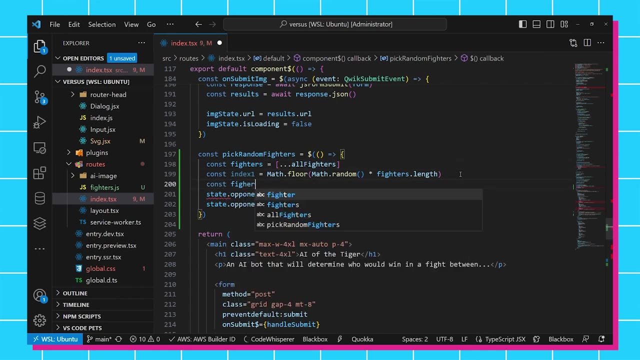 math dot random times, phi fighters, dot length, dot length. there we go. that should give me a random index between zero and the length of this array. then what we can do is say const: uh, fighter, fighter one, it's going to equal something. and again, what i want to do is essentially pluck fighter one or pluck an item. 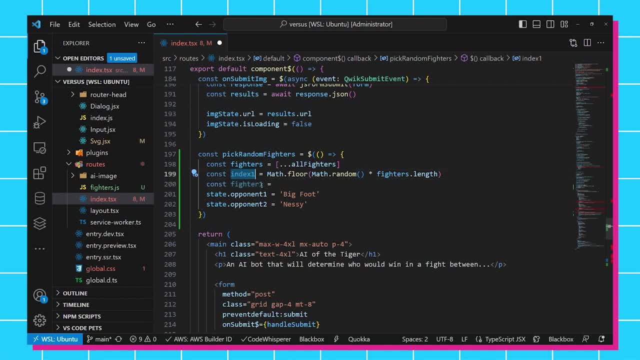 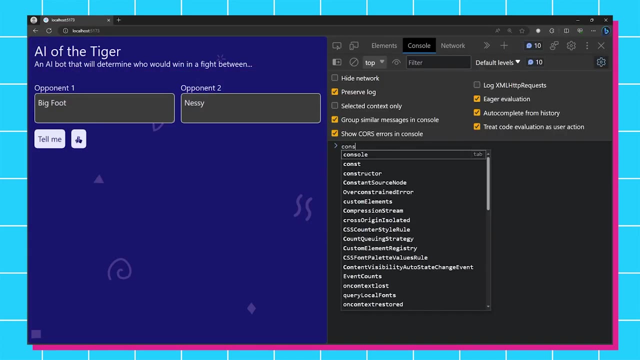 from this list at this index. but i don't just want to grab the value, i want to actually mutate this array such that, uh, the item is removed from the array at the same time. so we can actually do that. uh, let's, let's do an example in the console. so i'm going to say, uh, const array equals, and we'll do. 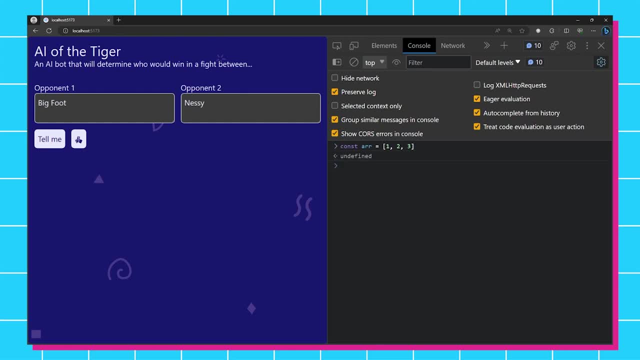 one, two, three, and then we can use splice to say, uh, let's see ar dot splice. and the way splice works is. it asks you at what index do you want to start? so let's say at the second item. we'll take one represents the index of the second item. and then it asks us which number of items we want to. 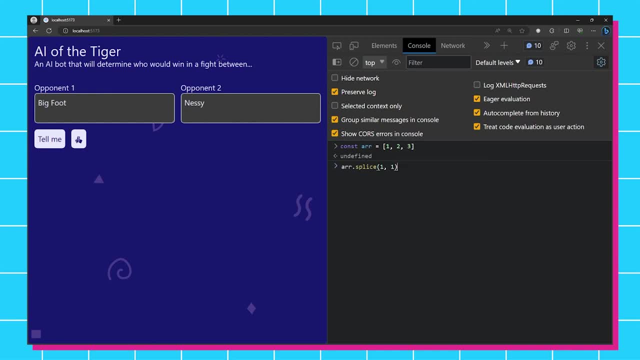 delete. so we want to remove one item from the list. we can do that. so array dot splice- uh, one one. and then what happens when i submit this is we're going to get an array back. so this actually returns an array with the item that has been deleted. so now we can see: array dot splice. 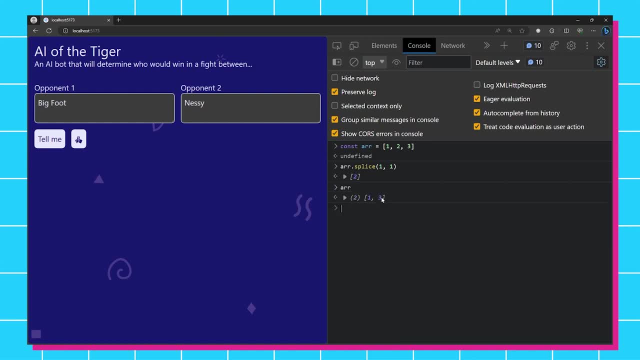 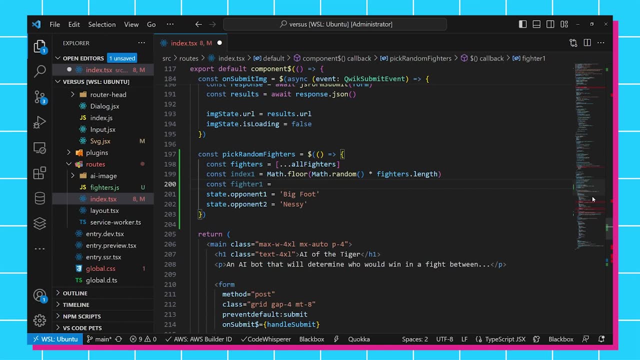 returns the number two and if we look at array we can see that it is left with the number two and number one and three. so this effectively does what we want. so we can say, uh, fighter one is going to equal fighters dot splice. and then we want to provide the index which we have as index one. 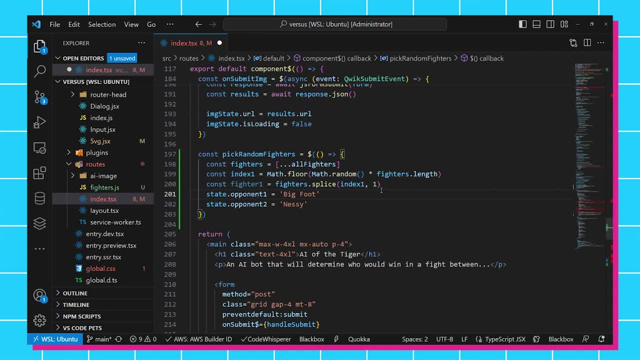 and then we want to provide the number that we want to delete, which is just one item and that's going to return an array. so I can either grab the first item in that array or I can actually destructure this call and say: uh, fighter, one is destructured from the array that is returned when. 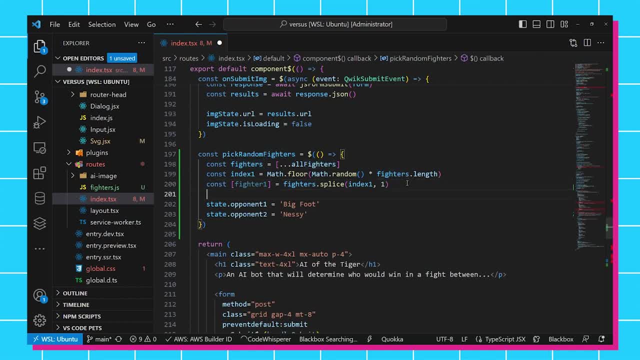 it's deleted and that, of course, is going to mutate the fighters array, which means that from here we can say const index two is going to equal, uh, essentially this same exact line, because now we're working with the mutated array and of course this is probably a good one- to uh turn into a 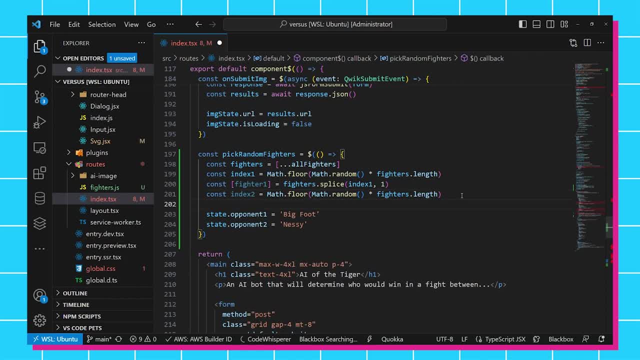 utility function. but I'm not going to do that today. but this does mean I can say const fighter two is going to equal. and now we don't have to do this splice. we can just randomly select an item from the array because we don't need to mutate the. 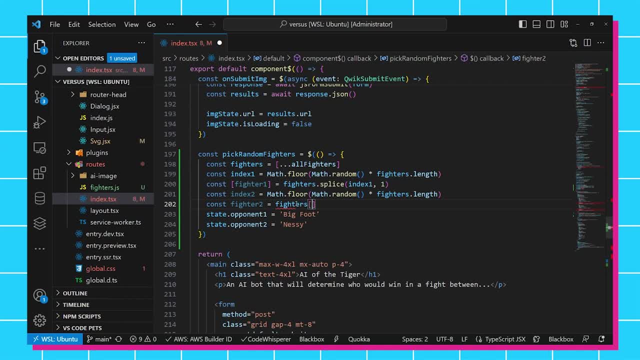 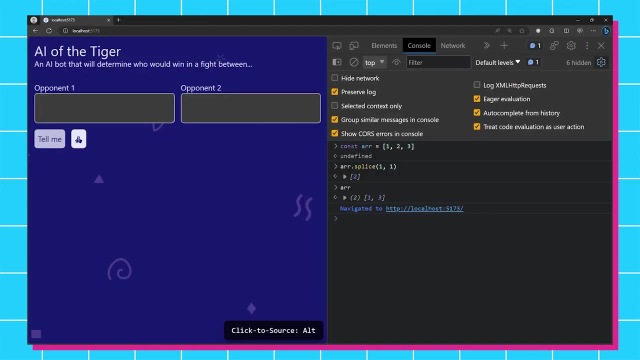 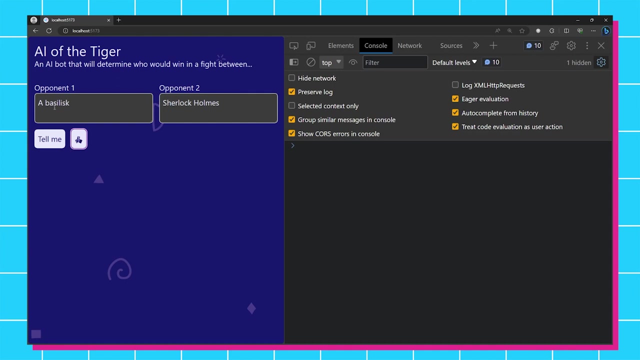 array. so now we can just say fighters at the index two, cool, that gives us fighter one and fighter two, which means I should be able to come here and do that and do that and replace that with two: fighter one, fighter two, and let's see if this works. all things, all things lucky, uh boop. hey, look at that. 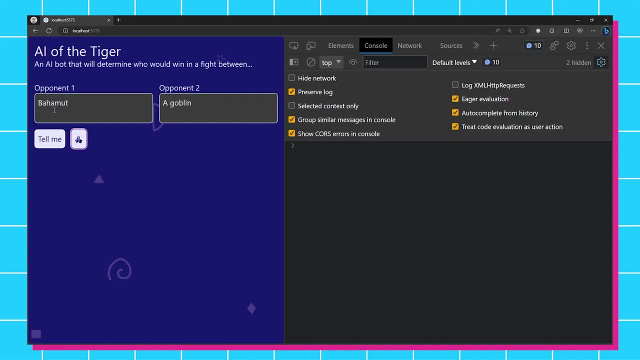 uh, a basilisk versus Sherlock Holmes. we do it again. we got Bahamut versus a goblin. we do it again. we got a ninja versus Cthulhu and Zeus vampire. here we go. what are we going for? we're gonna do a Viking versus a dragon. we're gonna tell that, or ask it to tell us. there we go, of course, a dragon is gonna. 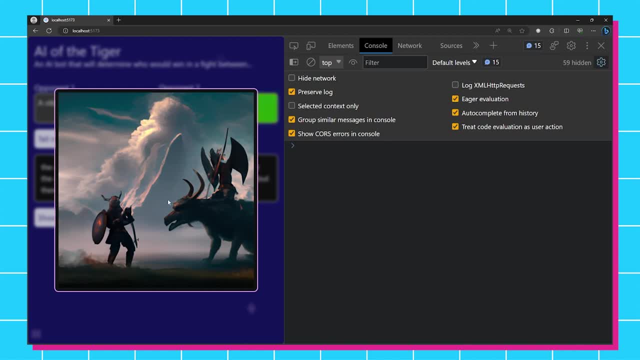 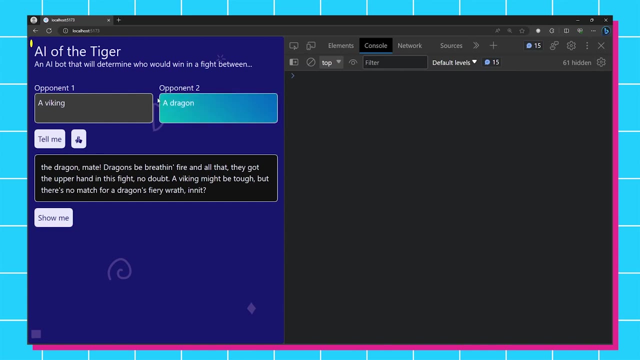 win. but I gotta see, and here you go, really funky looking dragon, funky looking, uh, Viking, pretty epic background. looks like he's got a little buddy for some help on his back, so I don't know, kind of unfair fight, if you ask me. okay, one more thing we need to do here is we probably want to reset the. 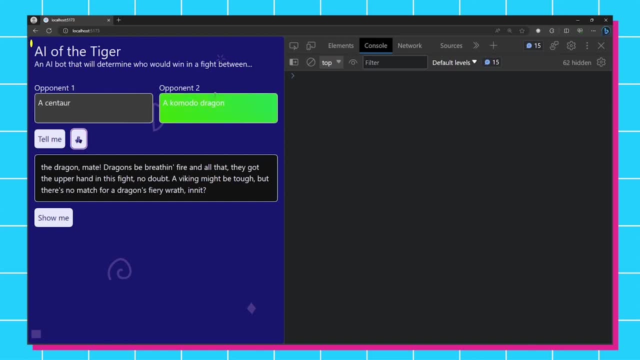 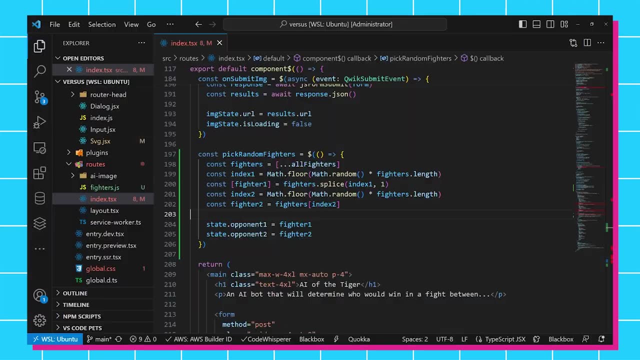 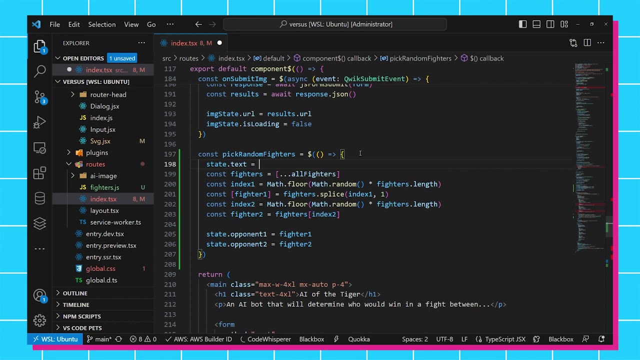 state of the app when someone clicks this. because if I click it again, we can see that we still have a winner selected, we still have the text here, but we are changing these inputs, so let's implement that as well. pretty simple, let's just do it at the beginning: uh, state dot and we'll say text is reset. 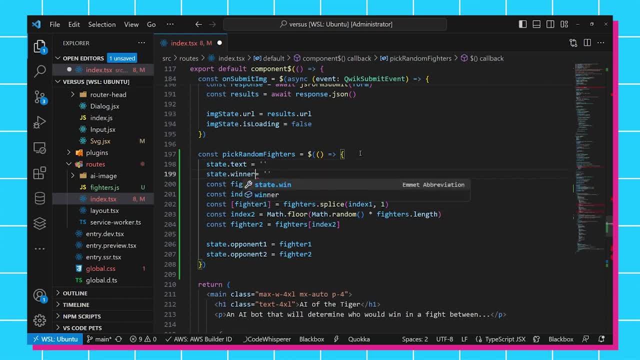 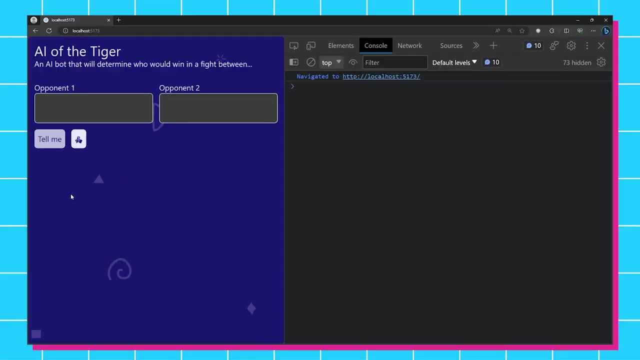 and same with the winner. reset that, then we do our logic, then we assign it. looks good to me, okay. next thing I said I wanted to do was mention to people that are using the app that, hey, things might look a little wonky like that dragon and 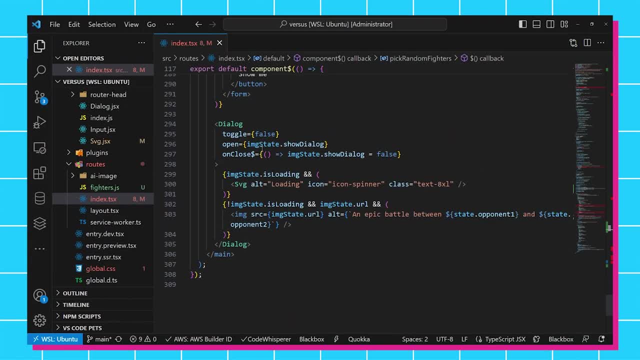 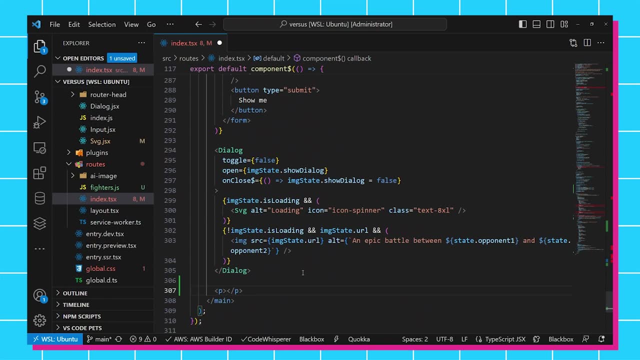 Viking, so I'm gonna go down. this is just in the template somewhere here. uh, let's yeah put it kind of here at the bottom. I'm gonna add a paragraph that says: uh- disclaimer: this app uses AI to generate content. so things may come out a little, a little wonky sometimes, and I think I want to give that some, some spacing. 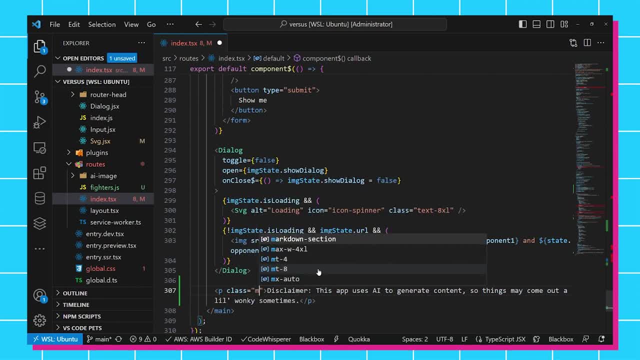 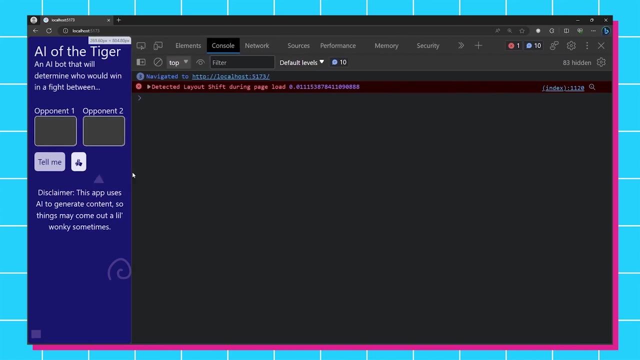 so we're going to say class equals, uh, margin, top and top and bottom like 10, and we'll say text Center. so let's see what this looks like. burp, that looks pretty good okay. um, yeah, that's kind of close on larger screens, so I'm going to give it a little bit more text on. 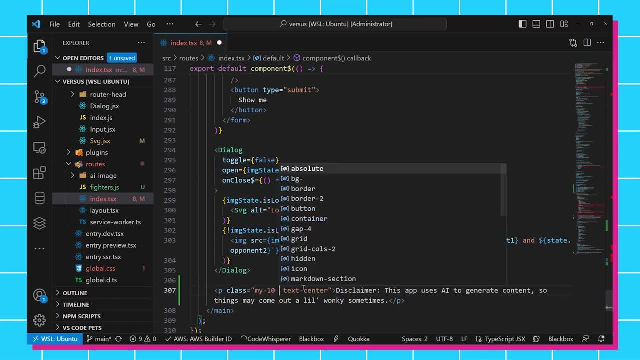 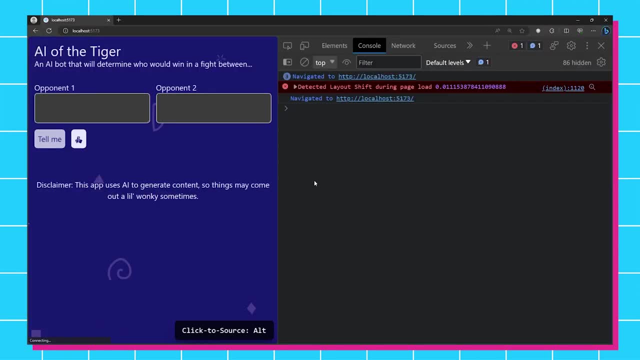 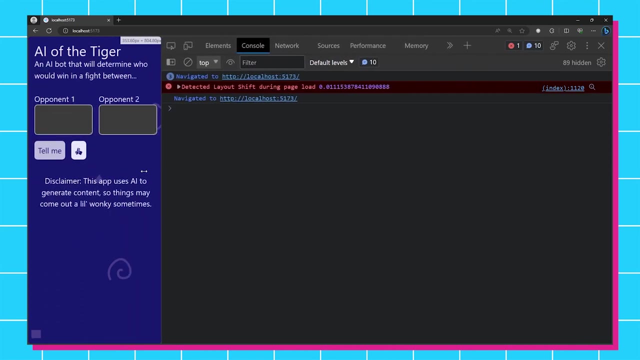 a small screen. so we're going to say standard is that, and then at the small breakpoint we're going to give it a margin top of 20.. there we go, a little bit close on small screens and a little bigger on big screens, and that actually gives me- it brings up a point that we didn't do- the spacing. 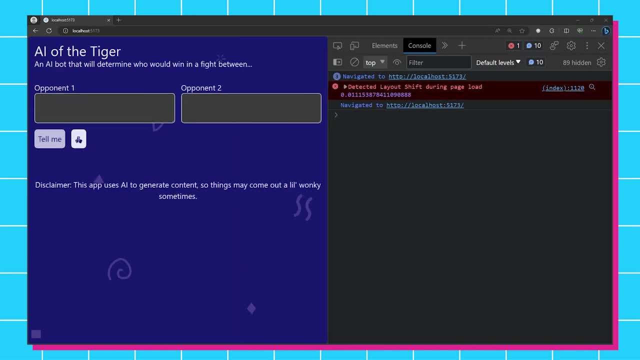 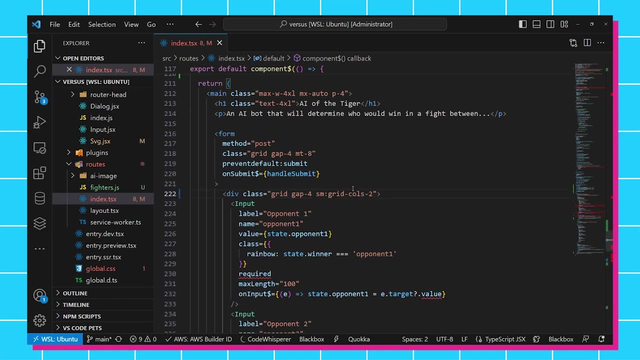 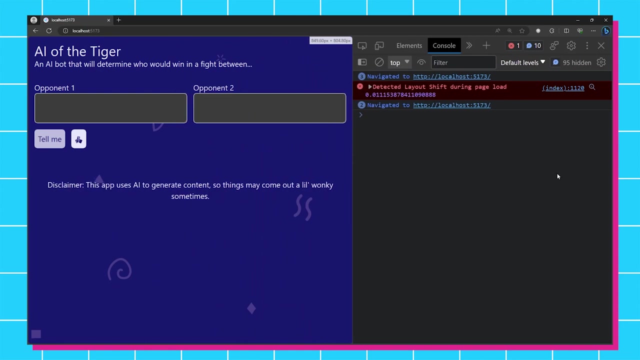 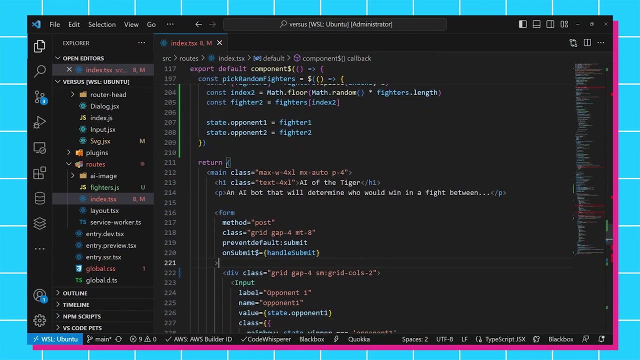 for small screens on that. so let's fix that really quick. here we go. no, where is it my inputs? uh, we only want at small breakpoint to go to two column grid. so there we go. looks good, happy with that, okay. last thing I want to do before we launch is I want to add a little bonus or a footer at the bottom of the page and 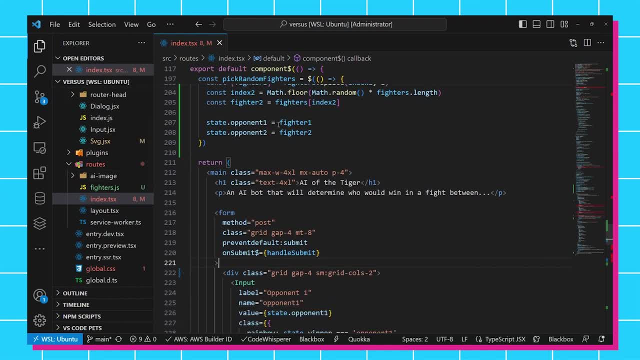 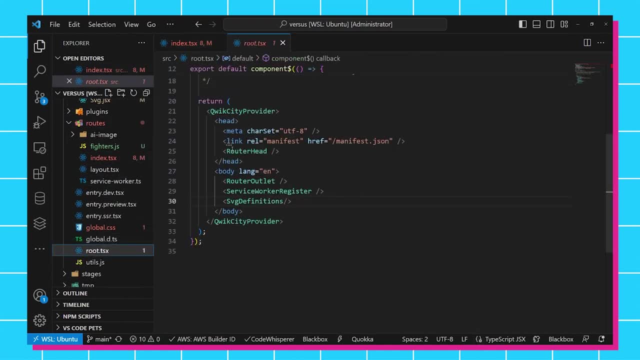 I wanted to cross the entire app. so instead of just doing it, uh, in this page, I'm going to do it at the entire app level, in the root component. so here we've got the head, we've got the body, uh, inside of my body. but probably before these things, I'm going to add: 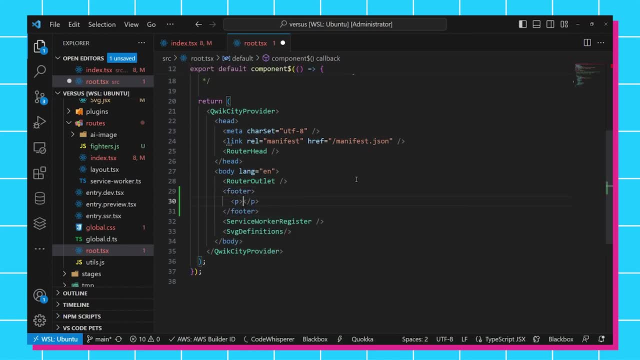 a footer and inside of my footer we're going to have a paragraph that says: built by: give a shout out to myself: slash austingillcom. because I'm super vain. we're gonna say: Austin Gill, there we go, uh, period. but it's also powered by. I'm gonna give a shout out to HTTPS colon slash. slash Akamaicom. 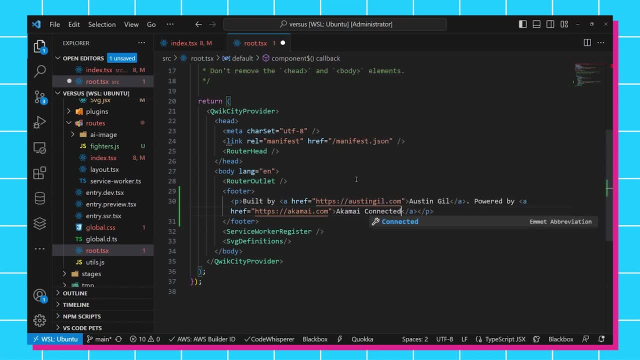 and say: Akamai, connected cloud, throw a period on there and then we'll have another paragraph. to spread some love, we're going to make this a whole link itself. you know, if you go to HTTPS colon slash, slash, lino, linocom, slash Austin, Austin, Gill, that's going to give you a. 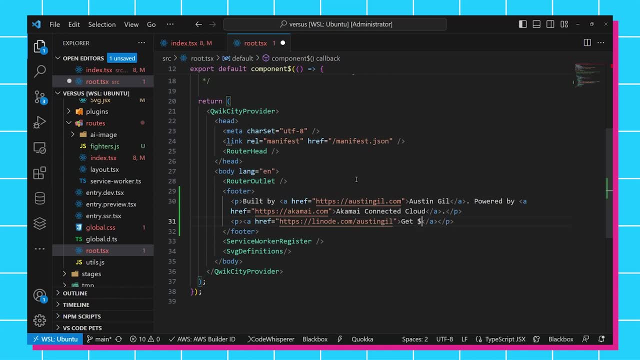 nice, a hundred dollars in credit, so get one hundred dollars in free cloud computing credits, baby, all right, how's that looking? uh not great because it's all there. let's add some styles to that. we're gonna go, uh, in the footer I'm gonna do a class equals. uh, give it some vertical and bottom spacing. 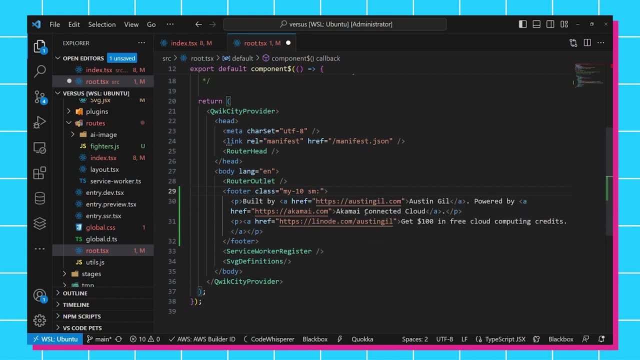 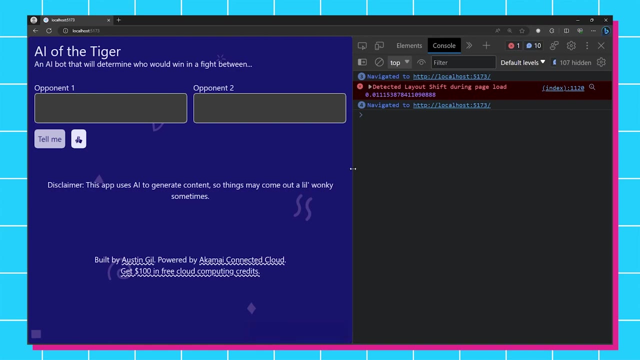 and then we're going to do the same thing at small screens: give it a little bit more and then give it some space around, so it's not right on the edge, and this is also going to be centered. so I think, if I got that right, uh, yeah, that looks pretty good. let's go small screen nice. 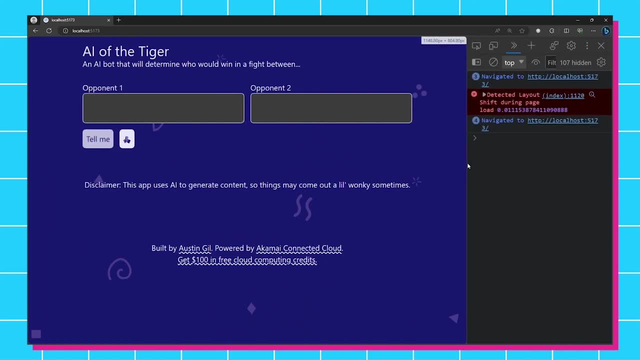 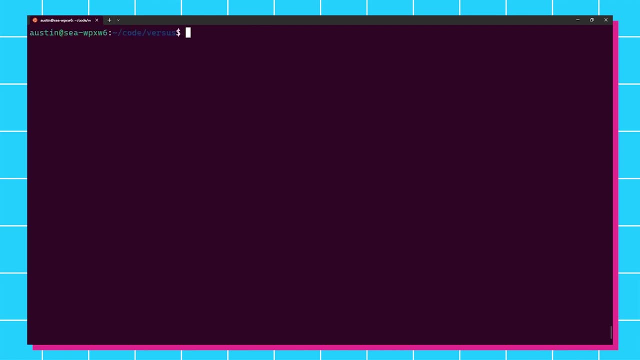 happy with that. all right, let's get this baby into production. so first thing we got to do is actually stop the dev server, because one thing that's special about quick is it's actually designed to run in multiple javascript runtimes, and that's handy. but it also means that our code as it is isn't ready. 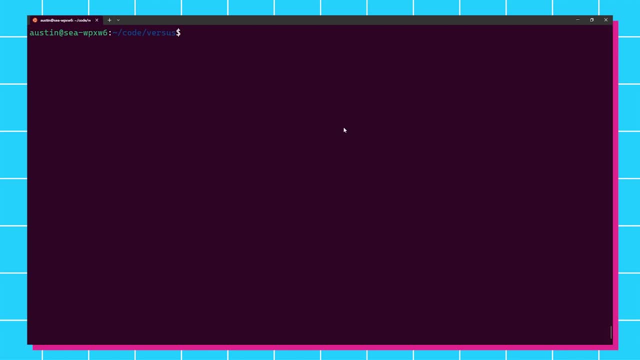 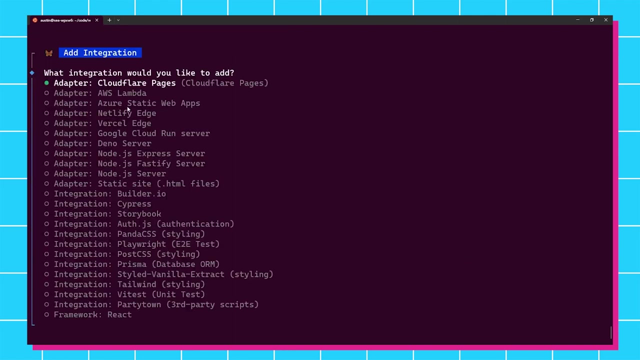 to run in production because it quick needs to know what the runtime is going to be, that it's going to run in in order to know how to run the code. so for that we're going to use some adapters and we can access them with npm run quick add, and this is going to prompt us with a whole bunch of 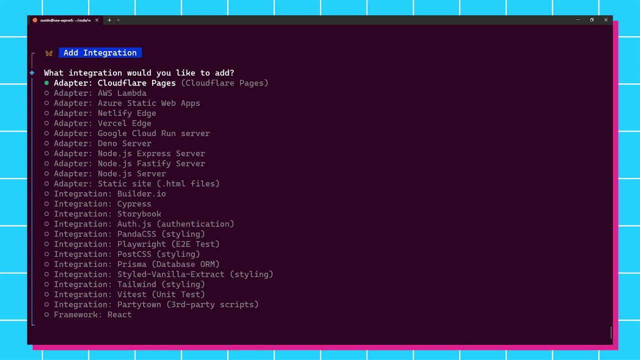 different adapters and integrations and plugins that we can tap into. so in this case i'm going to go down to the nodejs fastify server because i'm going to be deploying my application onto a vps running nodejs and i like the fastify server. if you see something here that you like, feel free. 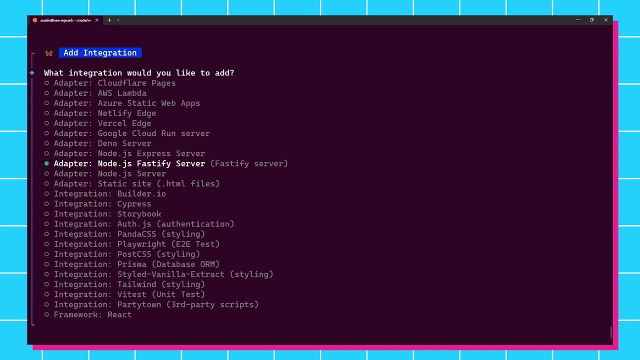 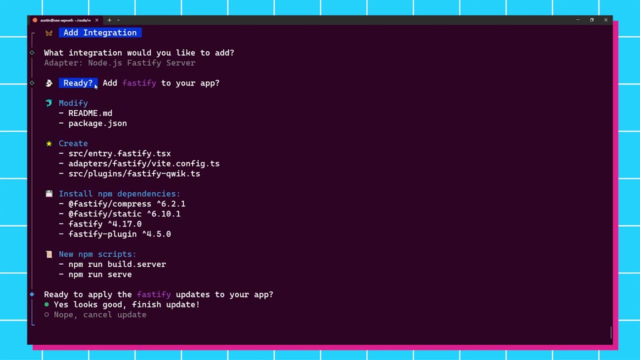 to choose it, but if you're going to follow along with me and actually deploy the app along with me, then we'll pick this fastify one. now, cool thing about this is it's going to prompt us with all of the changes that it's going to make, so it's going to modify a couple of files that are existing. 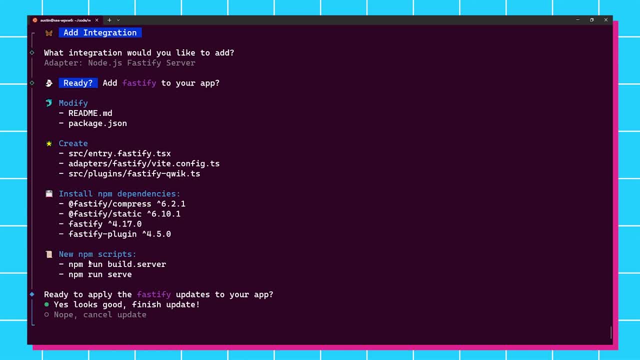 it's going to create some new ones, it's going to install npm dependencies and it's going to add some new scripts for us to run. so, as long as everything looks good, we can- uh, you know- choose between yes and no. i'm going to say yes, this looks good and it's going to run that script for us. 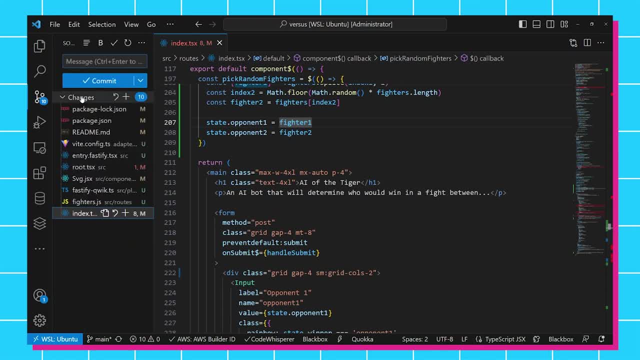 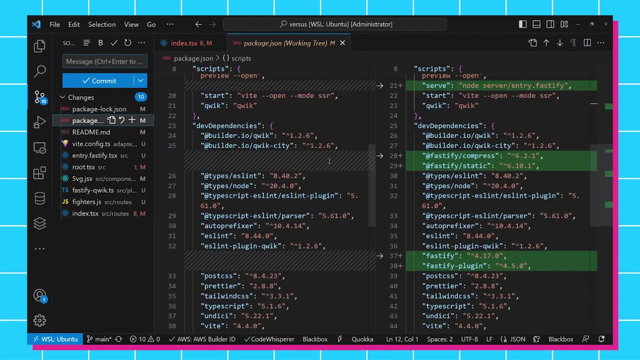 cool. so now, if we go back to our code, we can see that we have some changes in our project. now i didn't make any of the changes to the packagejson. we can see that those new dependencies are there and the new scripts. we can see that the readme even got a. 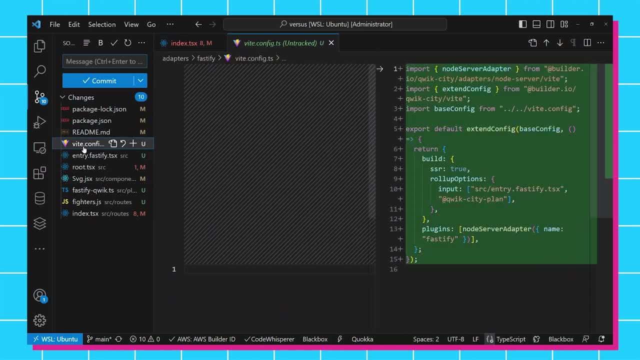 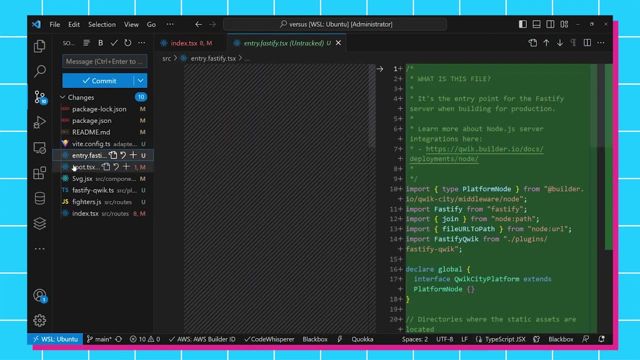 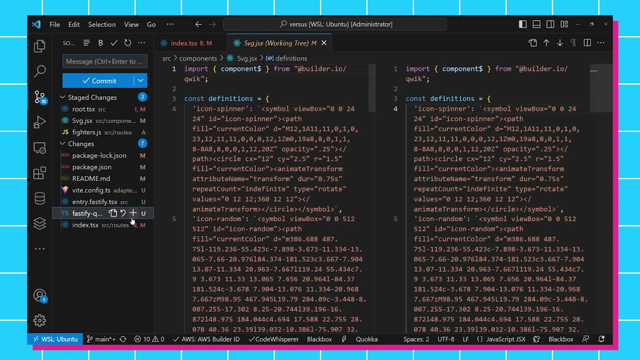 little better documentation, which is handy, a little addition of a new vconfig file for building our server, as well as the entry file to our server. this is the change that i made, so let's get rid of that. that is the change that i made, and then this is another change that i made. 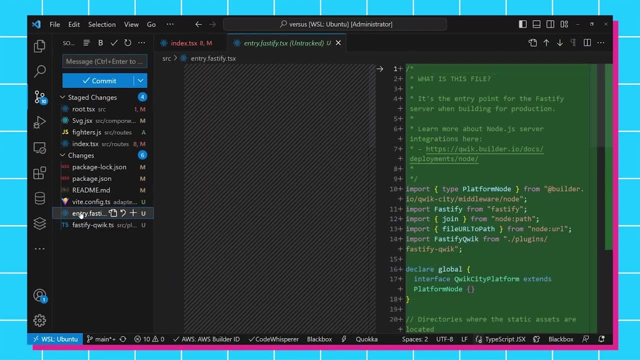 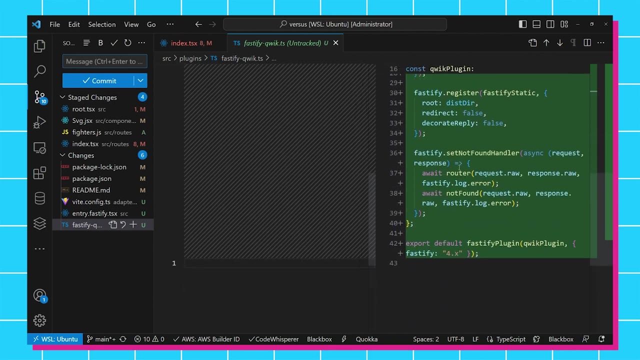 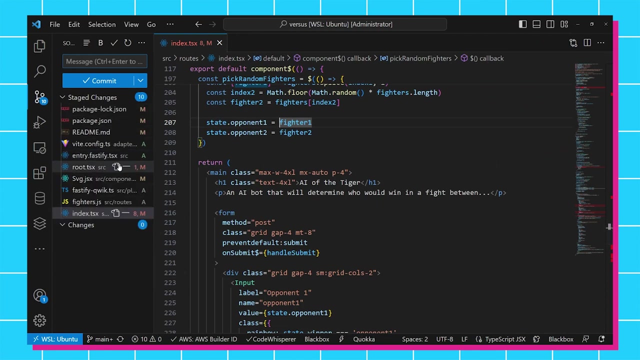 and that's a change i made. okay, outside of those, we also have this new entry, which is the server entry file for how to start the server-side app, as well as the configuration file for quick to instantiate the app in its specific runtime. so i'm going to apply all these changes. 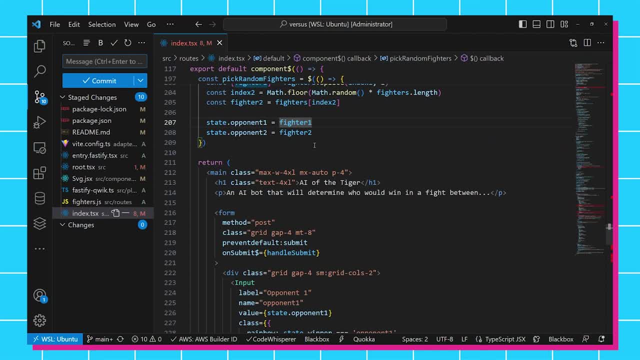 i'm going to push these up so that they are available in the repo, because i'm going to deploy this. i'm going to be pulling this, the all of these changes, down into the production server, so i'm going to say preparing for launch. all right, so let's push those. 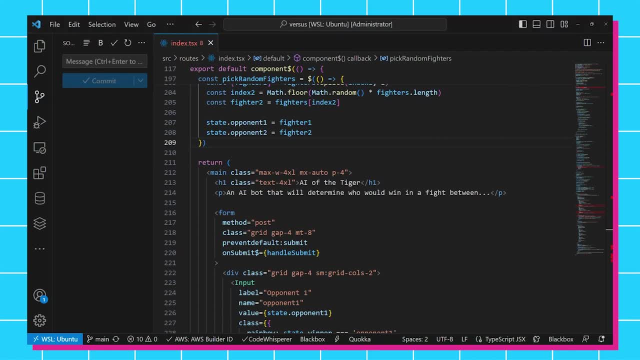 up. okay, sure, go ahead with all that taken care of. we are actually done writing code and we're going to shift to deploying our app in production. now, if you are going to be following along with me, you can head over to linocom. if you have not already signed up for an account, be sure to use my 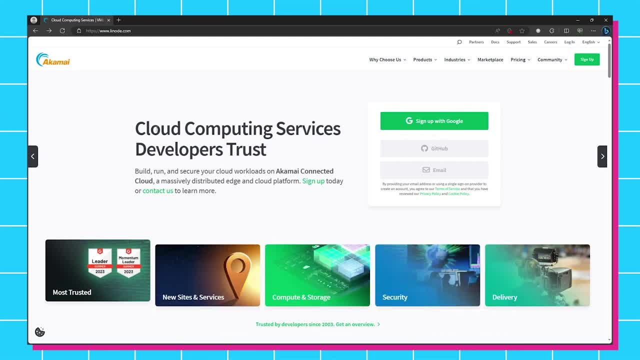 credits or my link to get some of the updates that we're going to be doing in the next few days. free credits: if you are not going to be using linode, that's okay. we are still going to be following standard steps that should apply to any vps service that you are using. but if you 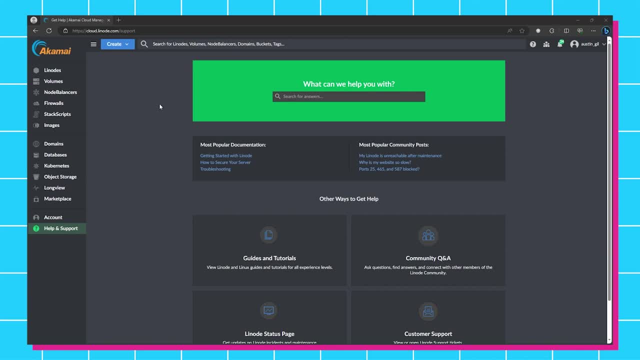 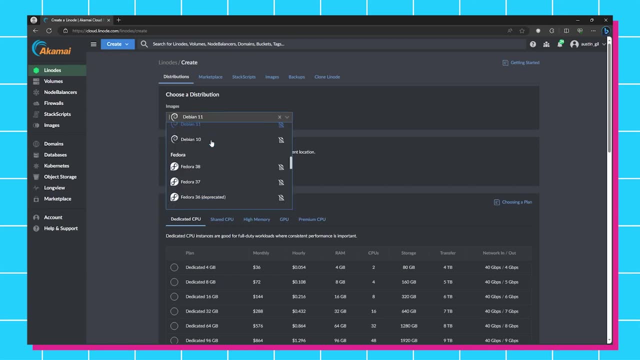 are using linode. assuming you have an account set up, then you can log into your dashboard and go ahead and create a new instance. now i am going to go ahead and use ubuntu, just because that is the operating system i am most familiar with. i'm going to use the lts version and i'm 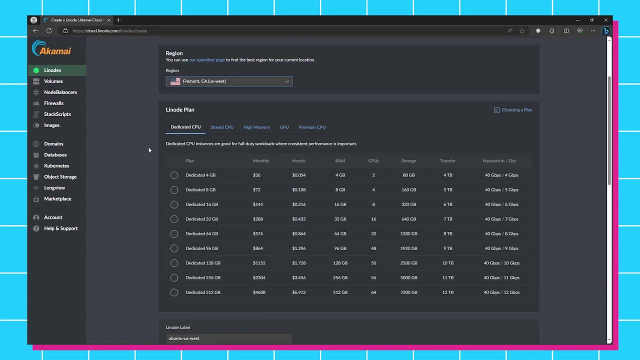 going to select a region close to me, because that's where, assuming, my users are going to be. for now, it doesn't really matter which instance you use. you can even use a shared nano one gigabyte, if that is what you prefer, and i'm going to give this a label. we're going to call this: 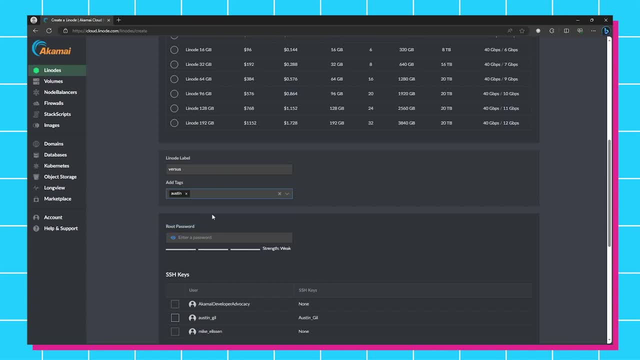 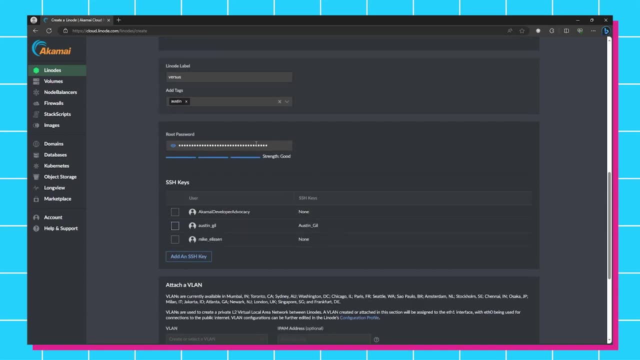 versus. i'm going to tag it as an austin creation and i'll give it a password. in my case, i'm just randomly generating a password that's really long and secure. i don't need to know it, because i have some ssh keys that i'm going to be using to log in to my system, so i'm just going to log in to my system. 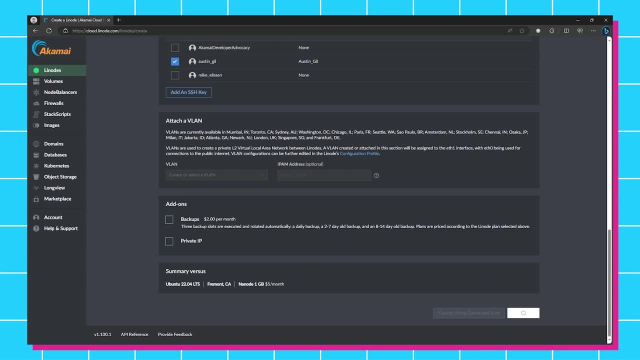 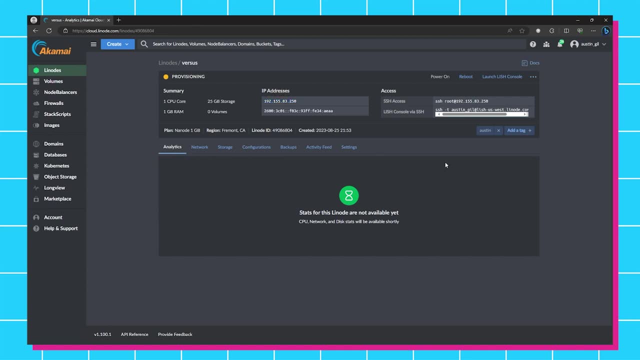 to my server. so with that all done i can create my linode, and this part might take a minute. so in the meantime it's a good idea to grab this ip address and go ahead and point your domain name to this ip address now. you don't necessarily have to, but it's going to be a lot easier if. 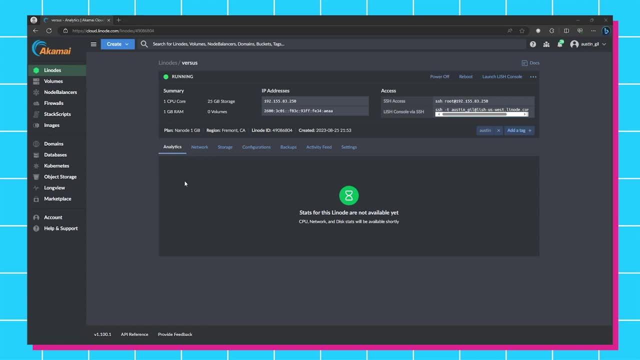 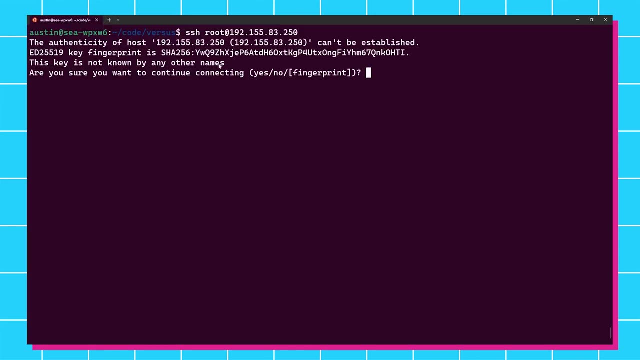 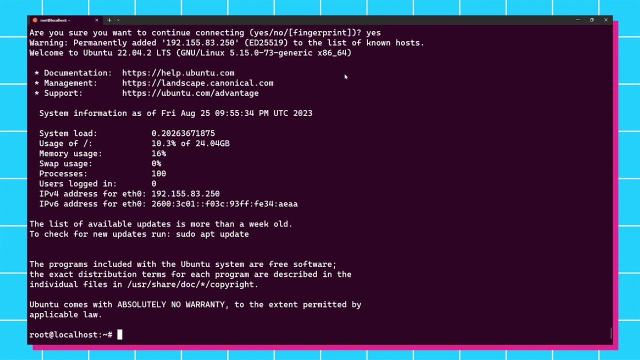 you already have a domain name set up. once our server is finished provisioning, we can copy this ssh command and go into our terminal and ssh into our server. and once again, if you have not, if you are not using ssh keys, there is a video that i show how to set those up, if you would. 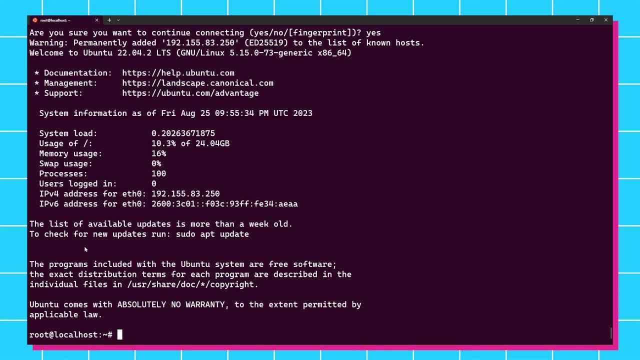 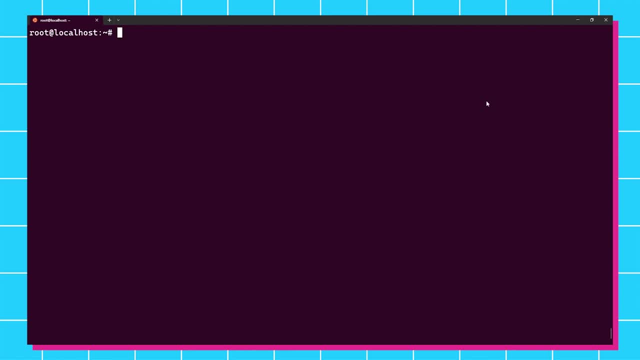 like to, but you will probably be prompted for your password. i'm using ssh keys so i just get right in, no problem. so the first thing we want to do on almost any server is to just update the existing software. then we're going to install git, then i'm going to go to 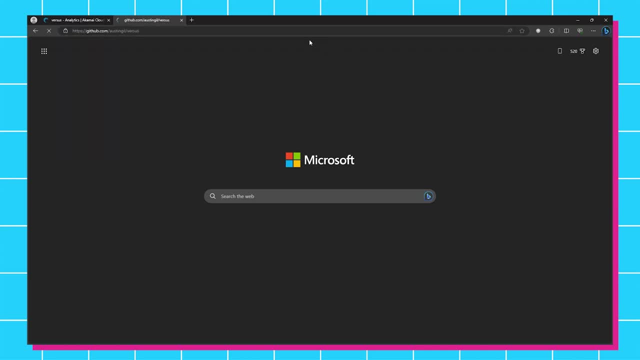 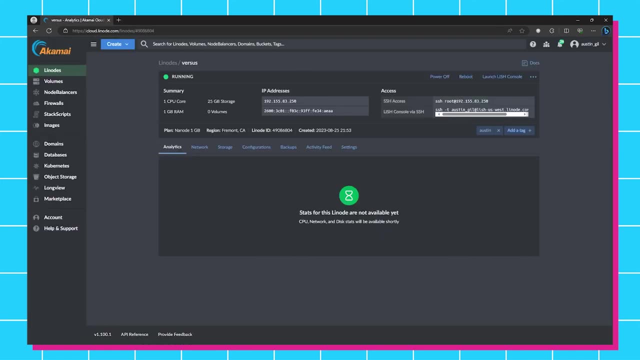 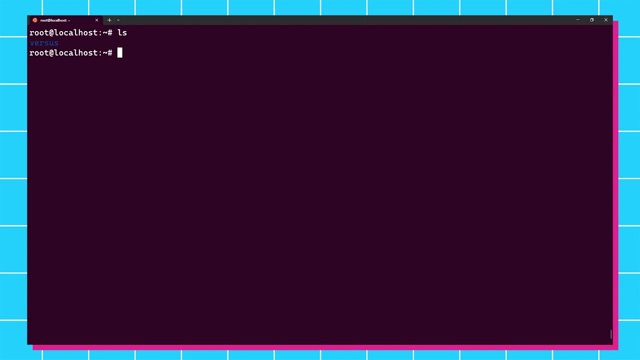 github, gil versus and i'm going to clone this project. so i'm going to grab the https version, copy that, push that down and then we're going to git clone. there we go all right, and with that we have the, the source code in our server. next i'm going to 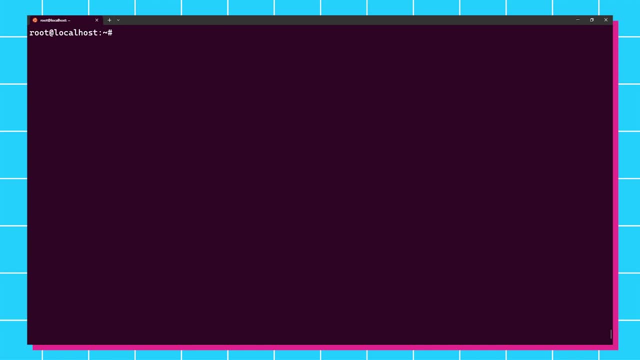 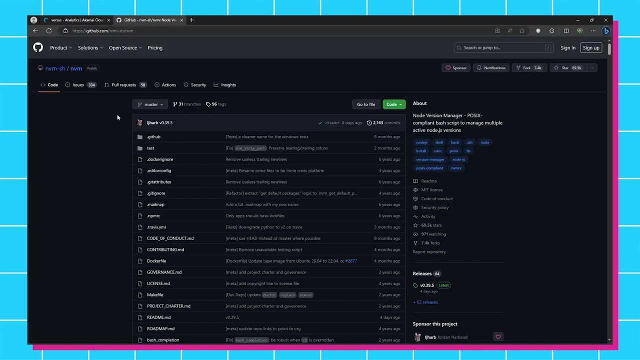 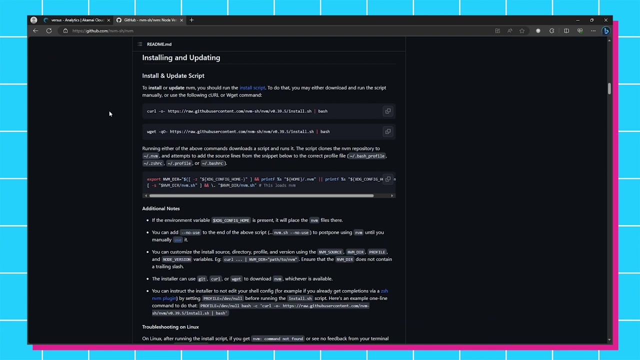 be running this application in a server that's running node, so we need to install node. i'm going to go. there's a project called nvm that i personally use and, like that, allows us to manage a whole bunch of different node versions. so we can go down to the install script and go ahead and copy that and paste it. 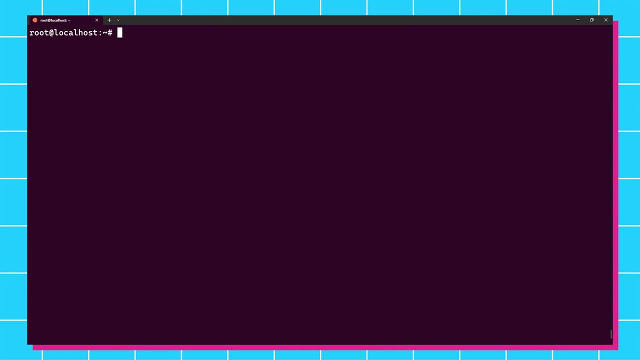 into our server and then we should have nvm available. of course, now if i type nvm, it's going to say the command is not found and you can fix that just by exiting the server and getting right back into it. so now if we say nvm, we see we have it available. 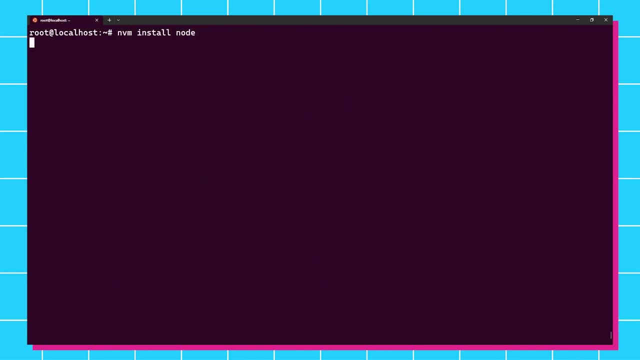 which means we can nvm install node- and that's going to grab the latest long-term release version, i believe- and once we have node, we also should have access to npm, which means we can get into our versus project and npm install the dependencies. okay, and once our dependencies are installed, we have to build the 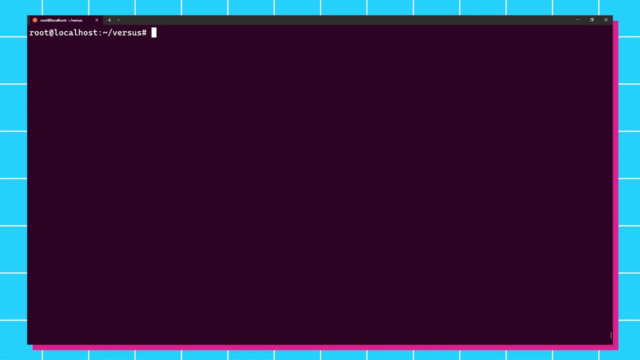 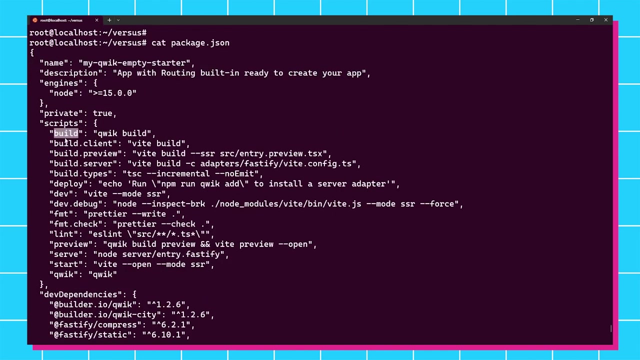 build the project for production. so if you remember, when we ran the npm run quick add and we added the fastify server, it modified our packagejson file so we can look at that if we want packagejson. it added a couple of scripts, including the build and the build server script. 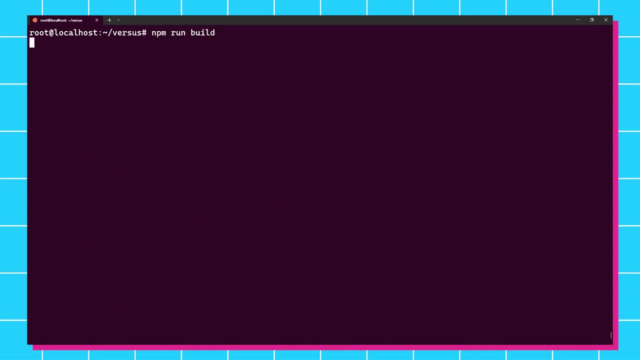 so we're going to actually run those. we're going to do npm, run build, and then this is going to run the build command and for some reason it builds the client, just fine, but it always hangs on the server for me. so we're actually going to have to run the server. 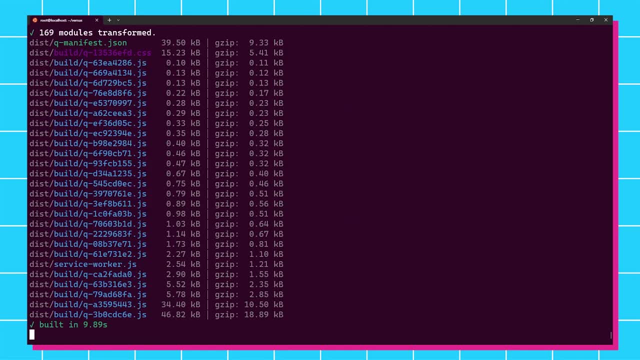 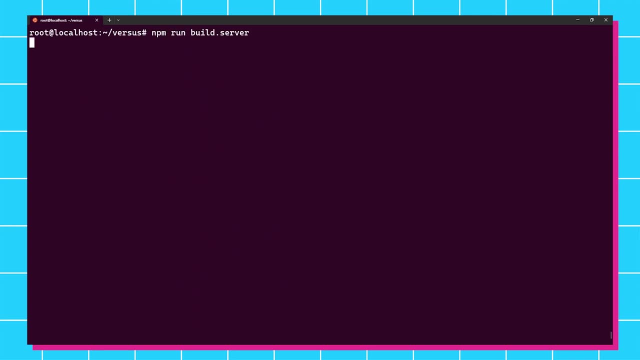 build script as well, and that is done should hang up, and then we can run npm, run build dot server and that's going to use veet to build the production version of the server code. all right, with that all set up, we should be able to run our application. but there's just one other thing that 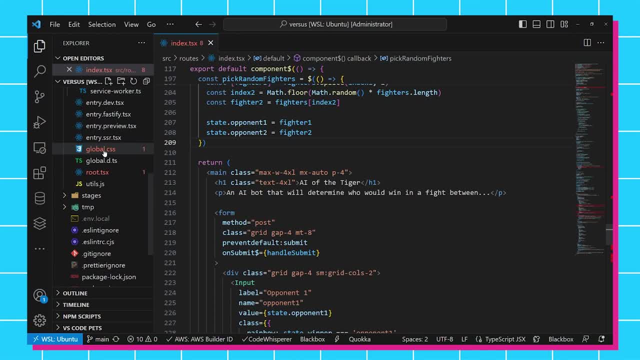 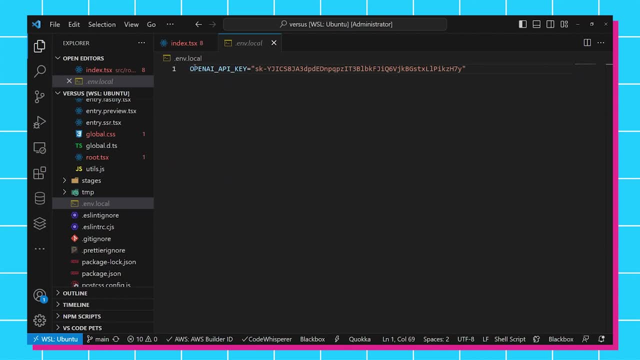 we need to be aware of. so, if you remember, in development mode we created this envlocal file that stored our environment variables and injected it for us. now, that's great for local development, but that actually won't work in production. however, we can take this code and 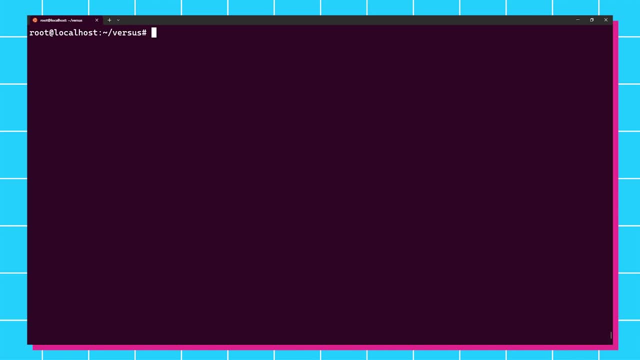 we can inject it in our cli as we start the application so we can copy that and paste it. and then we can start the app with npm run serve and we can see that that's going to call this node server entry fastify and then we can see that the application started running and started. 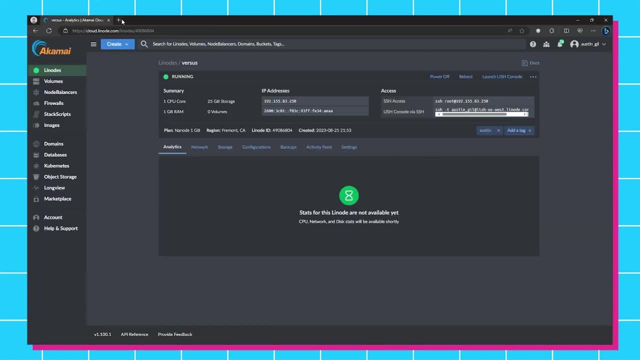 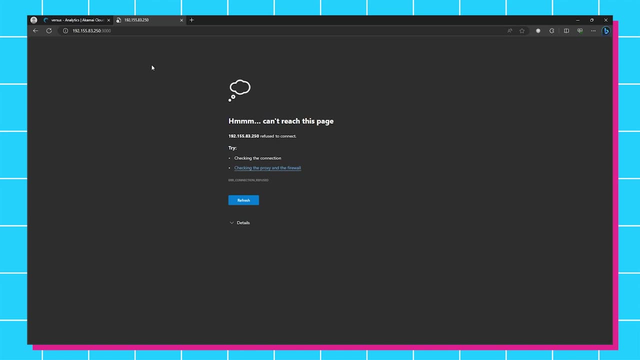 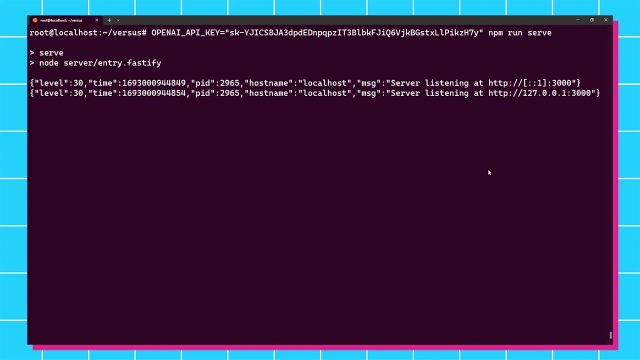 running the logs. however, if we go to our server's ip address and go to port 3000- because that is the port that fastify is going to run on- it's not actually going to load, and that's because we need to expose the port that it's running on and we also have this issue that the server is running. 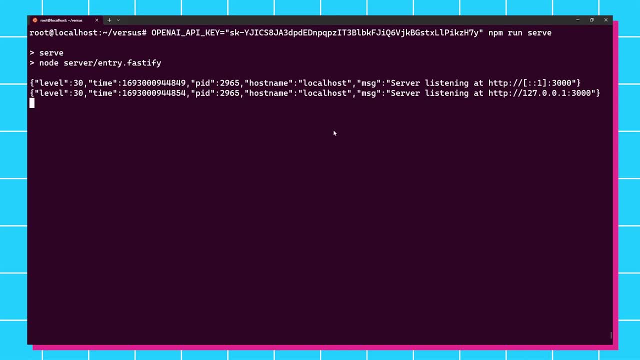 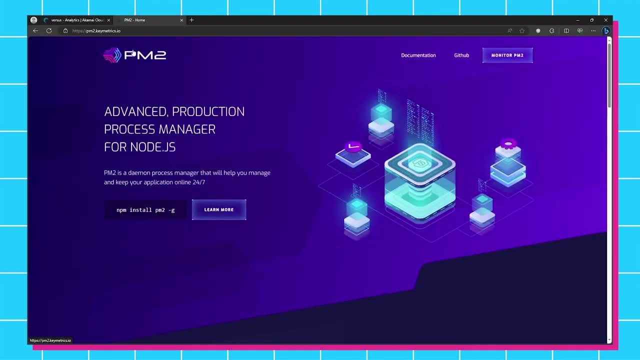 as long as we're logged in and waiting for this app to run, but if we want to exit out of the server, we end up killing the running process. so a handy solution for that is to use a project called pm2, which is essentially a process manager that can run your nodejs applications and make sure. 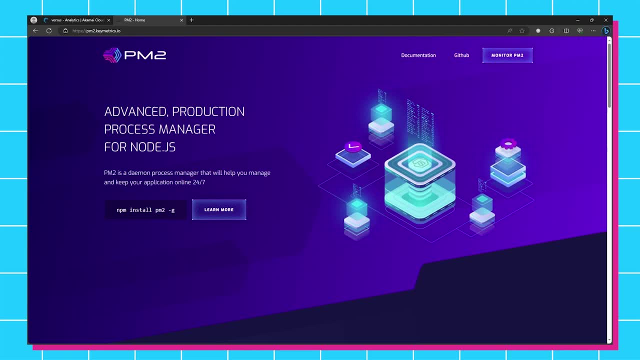 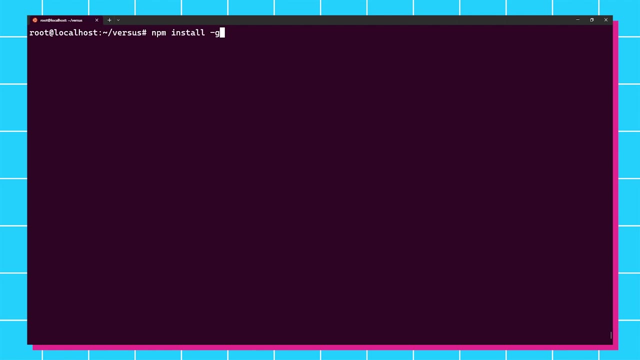 that they're using multiple cores on the server that they're running on or making sure that if it goes down it comes back up and in our case, it will run the process in the background while we exit out of the server. so we can work with pm2 by installing it via npm. so npm install as a global. 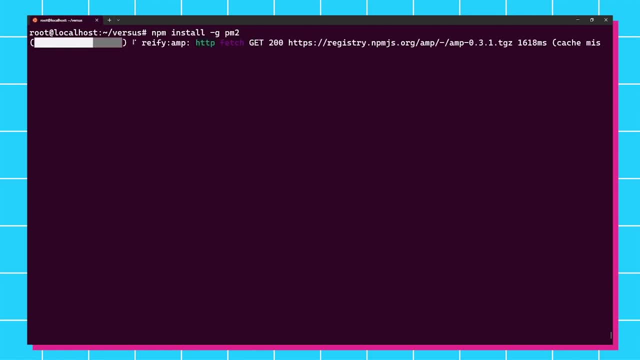 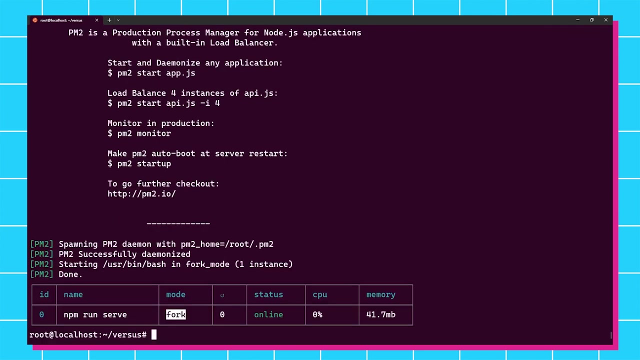 module pm2. so now we can run the same command but instead of running npm, run serve. i'm actually going to save that as in in a comment and right here i'm going to say pm2 to start a process that's going to run npm, run serve. if we do that, we can see that pm2 has done- uh, some pretty cool stuff it. 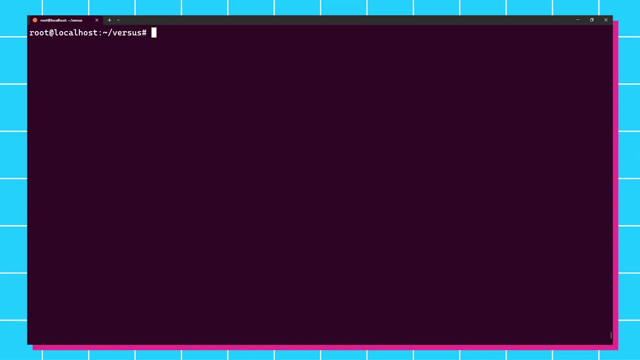 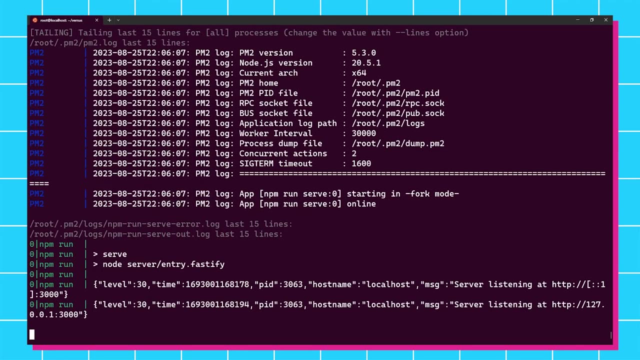 opened up our application and it's running in the background. there's a lot of handy things from pm2, like pm2 being able to uh log things and we can see what the server logs have been saying, as well as ensuring that if the server goes down uh and comes back up, pm2 will start the process. 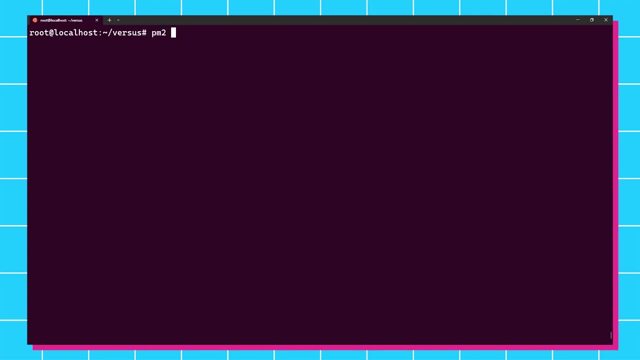 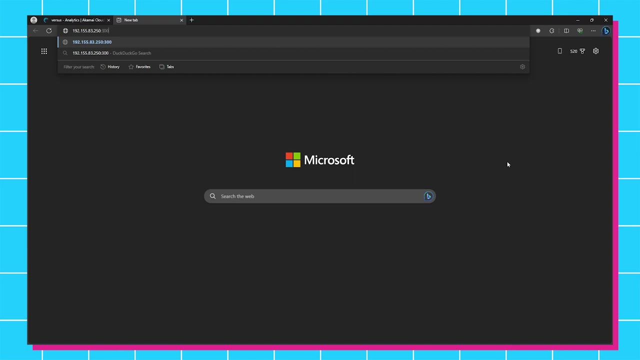 up again. uh, when it starts up. so we can do that with pm2 start up and that's going to generate a startup script for us. so now, if the server reboots, pm2 will be back on it. okay. so that's all well and good, but it still doesn't solve the problem of being able to access our server at our 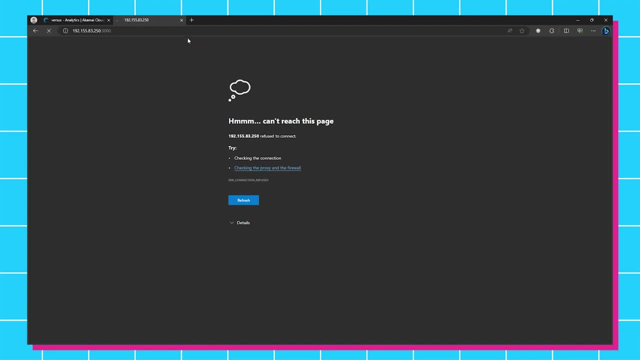 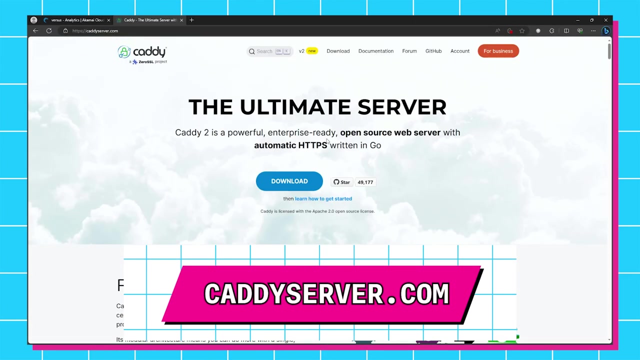 IP address and port 3000,. we still don't see the application running, And for that we're actually going to set up a reverse proxy using caddy server, caddy server server dot com. So this is a really awesome server that I've been using for a long time. It's built on go. it generates automatically. 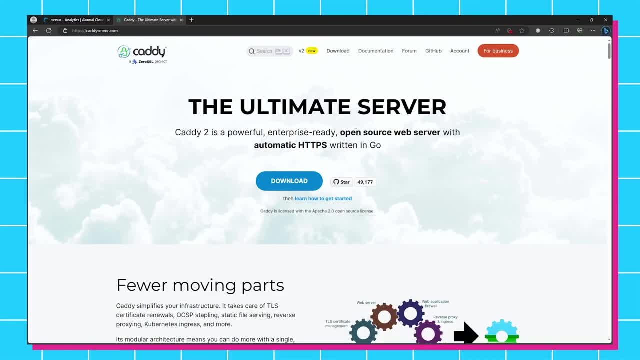 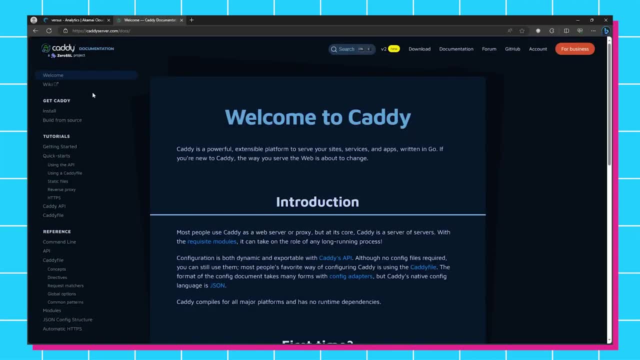 the HTTP SSL certificates for you and handles rewrites and can serve as a very good reverse proxy, which is what we want to do today. So we're going to go to the documentation and look up how to install it And we're going to scroll down, in my case, to the Ubuntu instructions And 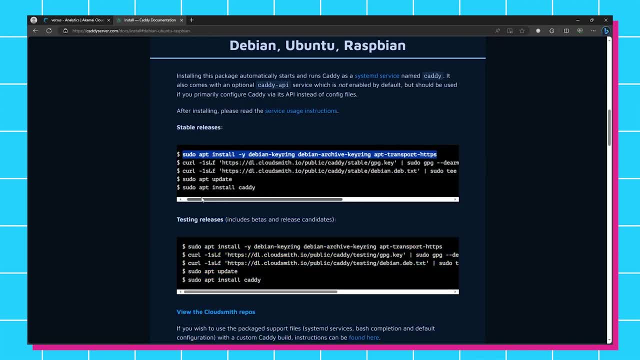 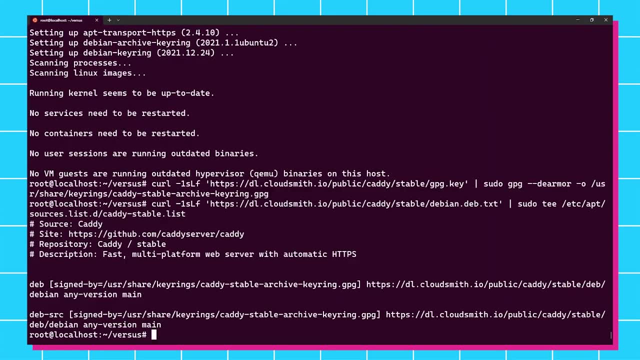 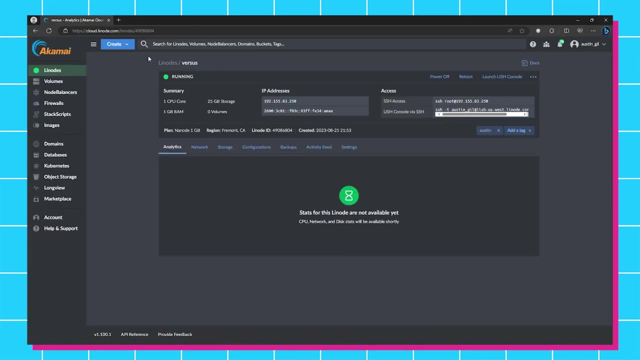 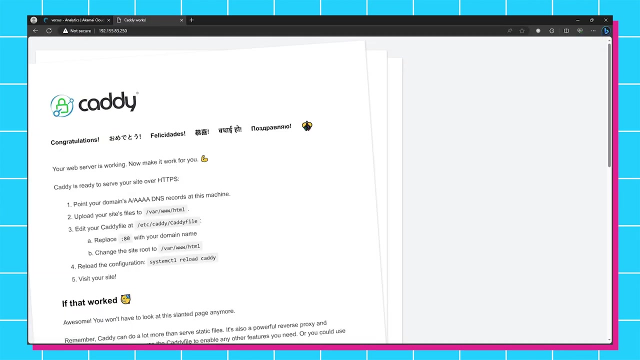 I'm just going to copy these commands and paste them into my terminal. So I'm going to copy that one and paste it there. All right, so now that caddy is installed and running, now we can go to our server's IP address And we can go to root and we can see the default caddy welcome. 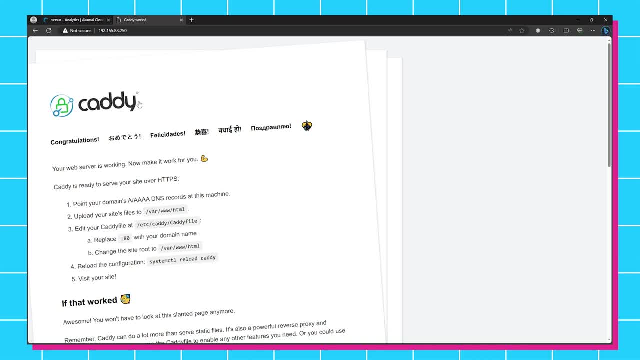 page. Now the last thing we're going to do here is we're going to use caddy to do a couple of things for us. I've already pointed the domain name versus Austin gillcom to this IP address. we just need to configure caddy to use it And once we've done that, we're going to have the. 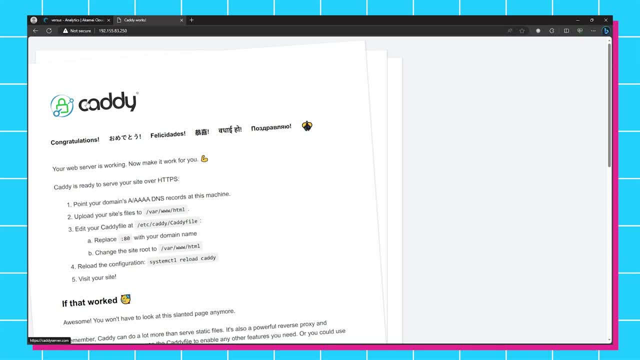 domain name be fixed. caddy is going to go ahead and provision an SSL certificate for us and make sure that it stays. We're also going to set caddy up to be a reverse proxy, So that our fastify server running at port 3000 will actually be at the root domain name. So we can see a couple of commands. here are examples: 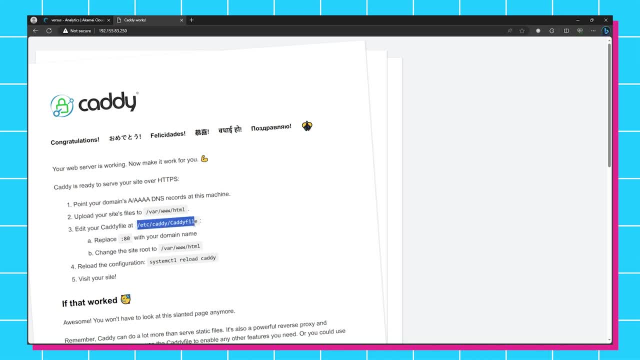 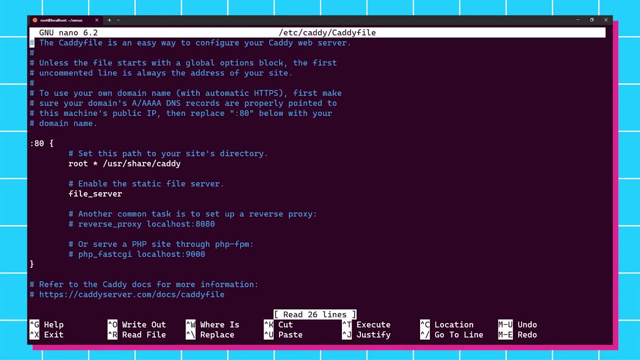 of what we can do And we want to configure all that in the caddy file here. So I'm going to copy this And I'm going to use nano- not mammo nano- to edit that file. So down here at this port 80,. 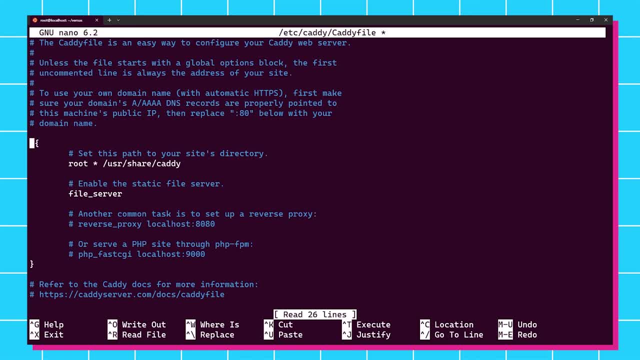 I'm going to replace this with my domain name. If you have not done this, if you've not done this, you can do that here, And then I'm going to go ahead and paste that ID. It says introducedors: So in was already been pointed at the my servers IP address, and then I 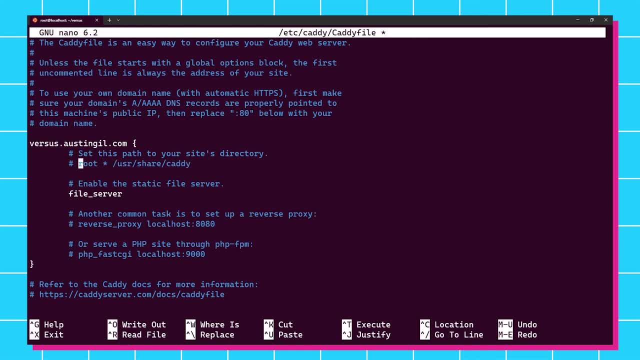 don't necessarily want this to be a static host, So I'm going to disable that And I'm going to- I think I'll leave the file server. actually don't know what that does, But I'm going to enable this reverse proxy And we have the reverse proxy running at Port 3000 when we're using fastify. 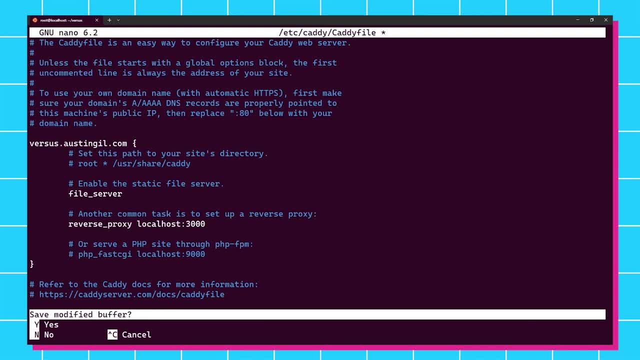 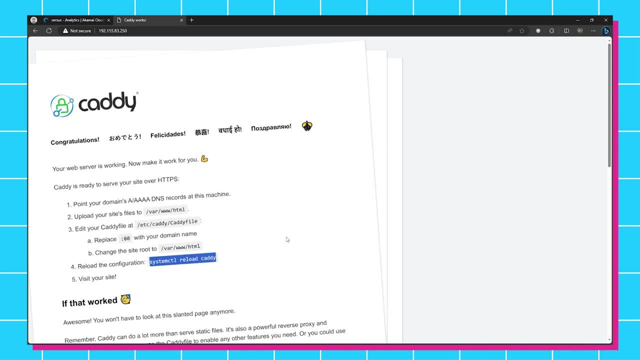 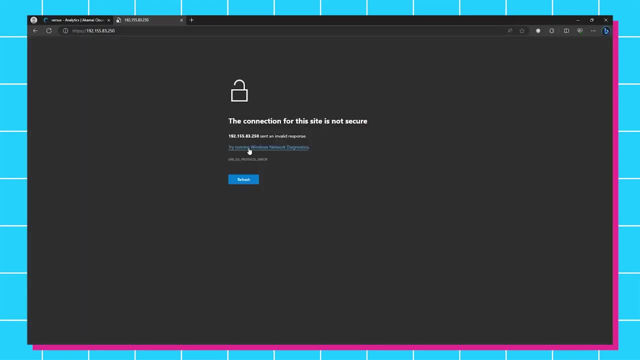 So I'm going to save that by hitting ctrl x and then y and then enter. now we just need to reload the caddy process so that it loads our new configuration file. and if i reload the application it's dead. but that's okay, because we didn't even run it running at the ip address anyway. what we wanted was to point it. 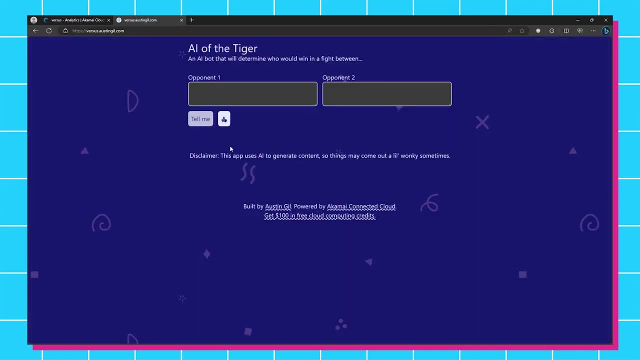 to versusaustinbillcom and there it is: boom shakalaka, it's our application that we just deployed and it's got the new features that we added. uh, and we can say: let's see a viking versus a king cobra, a rabbit squirrel versus a werewolf. okay, tell me how this one's gonna play out. 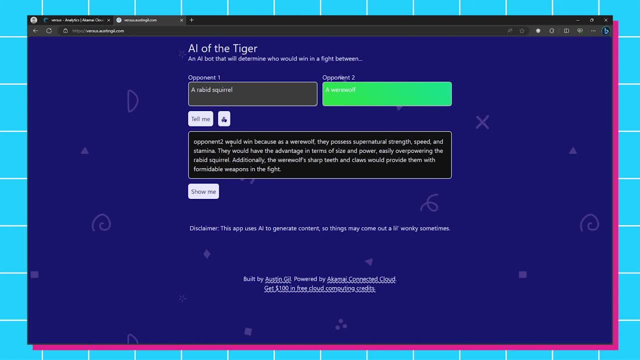 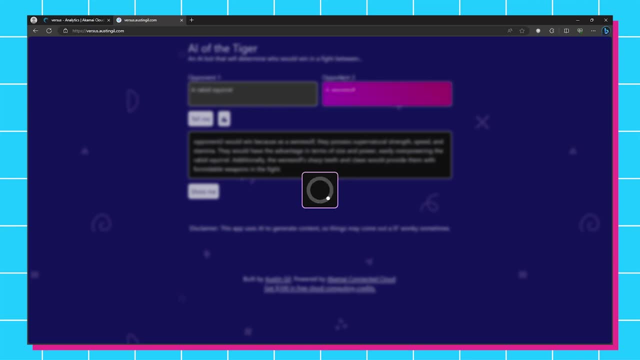 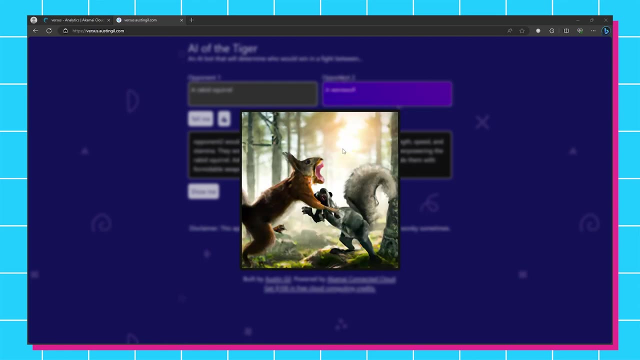 and we say opponent two. that's not what you were supposed to say, but it wins because it's a werewolf and it possesses supernatural ability. of course, a rabbit squirrel would probably kick my butt, but doesn't stand a chance. again, it's a werewolf. so there we go, another one of these uh wonky, uh ai generated images. this looks more like a. 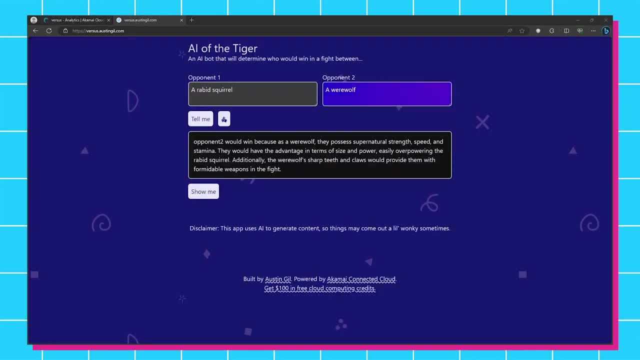 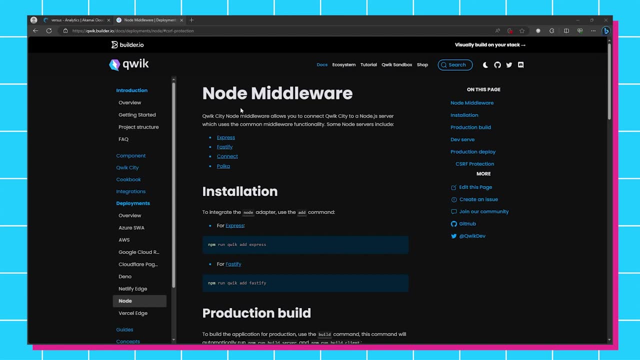 were squirrel, but you know, that's what we get now. there's one more thing that i want to point out here, and that is, if you didn't set up your application to connect it to a domain name and you did run it on some sort of node middleware, like, in our case, fastify. 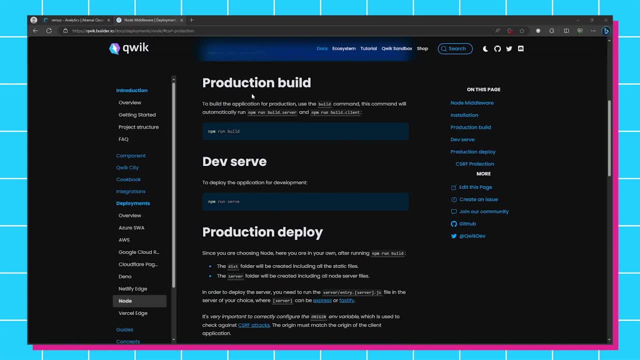 then you might run into this problem where, when you build for production, you're not going to be able to run it on some sort of node middleware, like, in our case, fastify, and you're not able to access your app using the ip address, even if you have the caddy server. 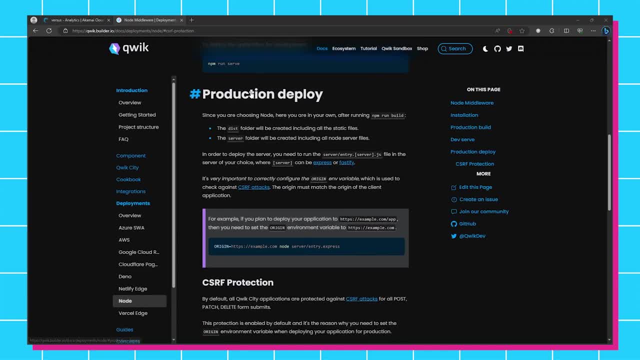 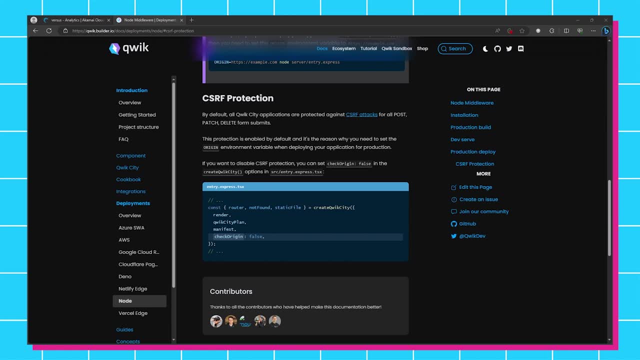 and reverse proxy setup, and that has to do with the way the production deployment works. uh, the quick team by default will set up csrf protection, which is really awesome to protect against cfrs- csrf attacks. however, by default that requires checking the name of the origin server or the url. so if you want to do that, all you have to do is set the check origin. 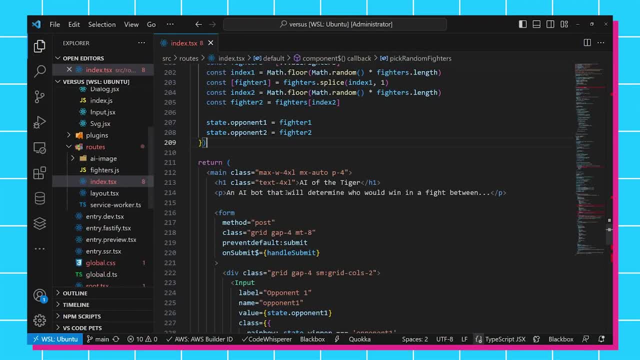 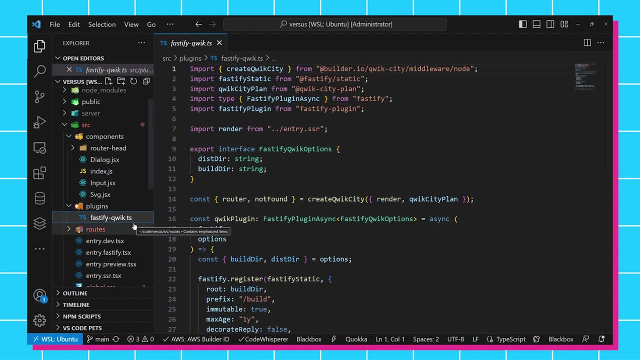 tag to false inside of your fastify configuration file, which should exist inside of source plugins, and then fastify quickts and it should be inside of this create quick city configuration. you can just pass uh, check origin and set that to false. now, of course, uh, you want to do this on the code. 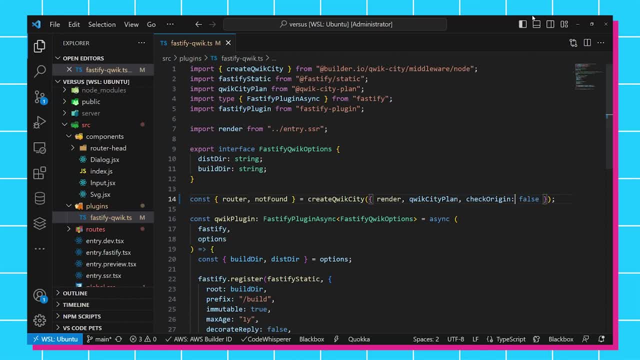 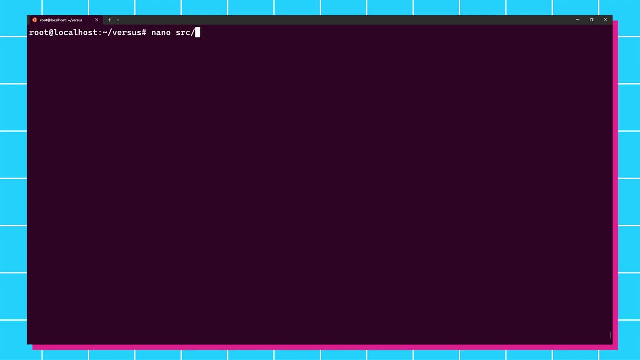 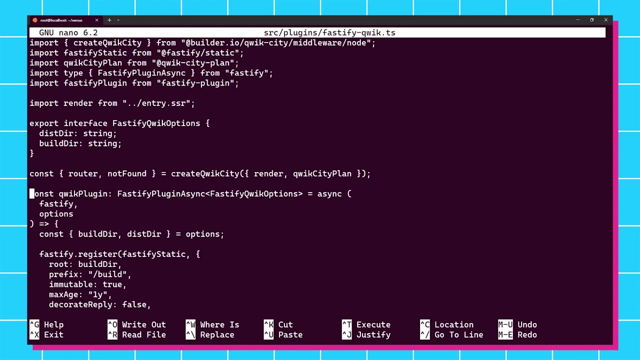 base that's in the server, so you would either have to push this to get and then pull it down to the server, or inside of your server you can modify the source slash plugin, slash fastify file and go down to the correct line and then comma check origin false and control x, y, enter and then 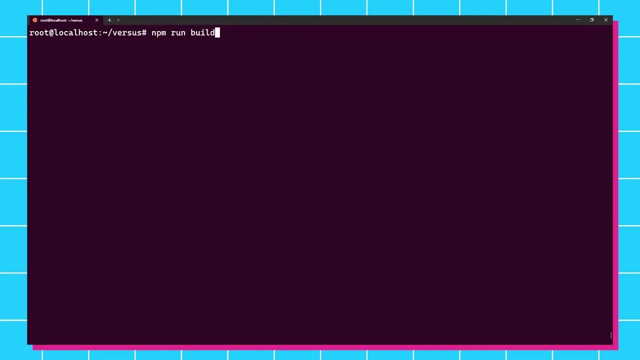 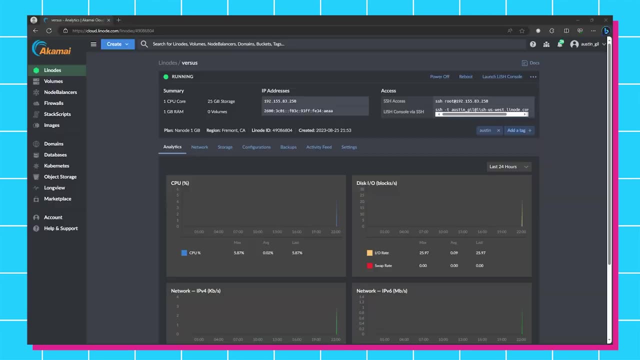 even after you do that, you'd have to run uh the build server command one other time, and once you've built the server you have to run the build server command one other time. and once you've built the server you have to restart the pm2 process. but once that is all said and done, you should be able. 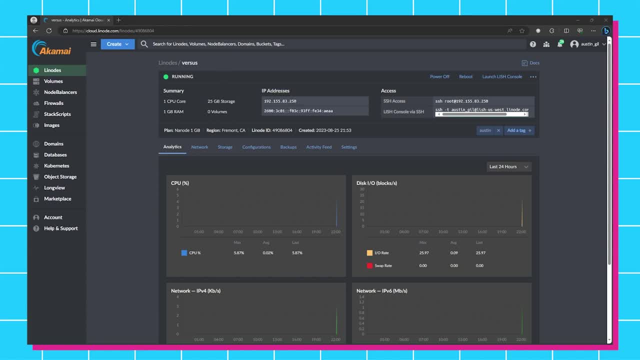 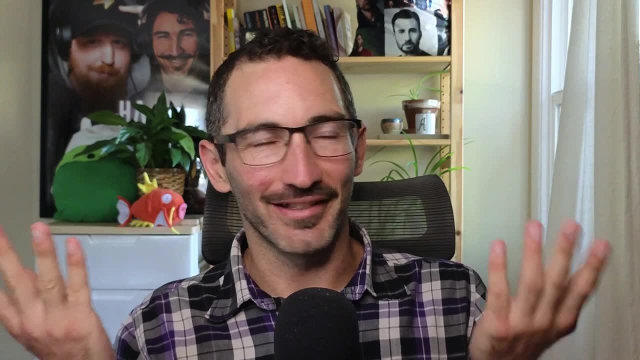 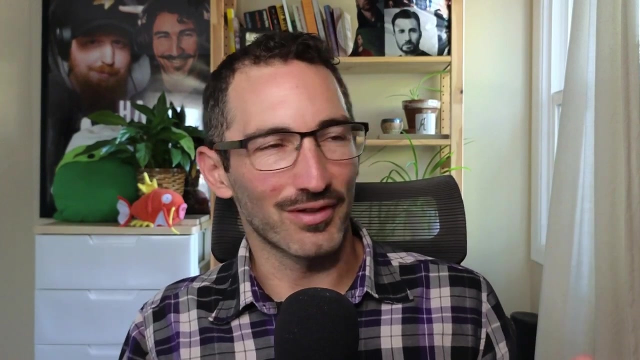 to copy your ip address, load it in the browser and see your application running. all right, it's working. how cool is that? you can go onto the internet in your browser and go to versusaustingillcom and get some silly uh fights and responses from ai. i really hope that you enjoyed this series.